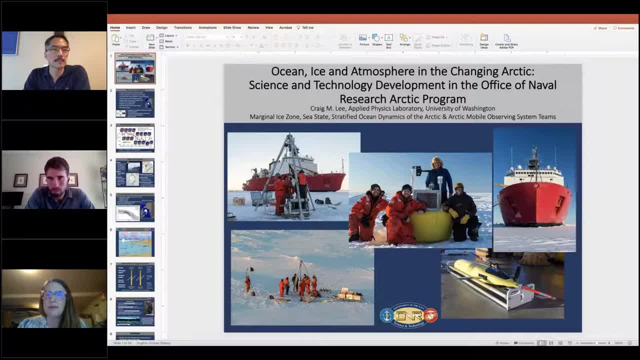 or regional issues in Alaska's marine ecosystems, And you can visit the EcoFOCI webpage for more information at wwwecofocinoaagov. So again, I thank you for joining us this morning as we continue this all-virtual seminar series. 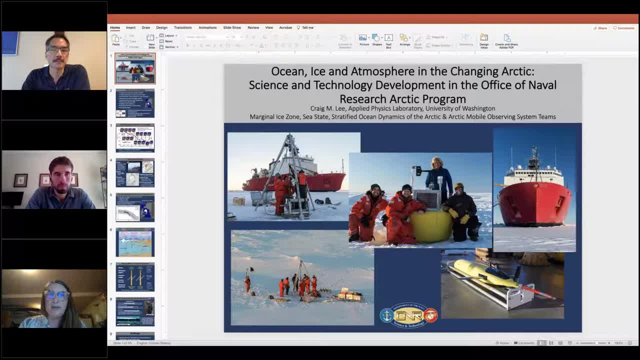 As I said, this is the last of our spring series. The fall is yet to be announced. In just a couple of weeks, most of our spring seminars will be posted on the PMEL YouTube page so you can catch them there if you missed any this season. 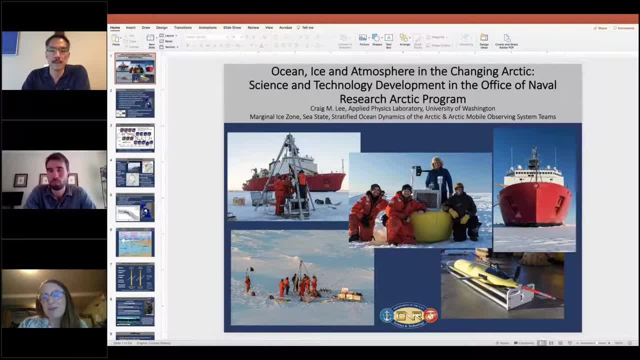 Please double check again that your microphones are muted, that you are not on video unless you're the speaker, and then, during the talk, please feel free to type your questions into the chat. Jens and I will both be monitoring that and we will address questions at the end of Craig's talk. 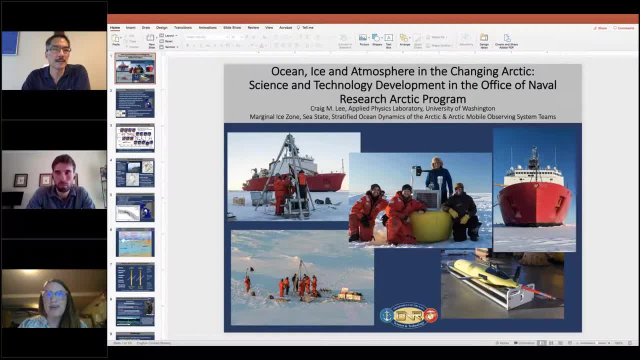 So today I am really excited to introduce Dr Craig Lee. He is a senior principal oceanographer at the University of Washington Applied Physics Lab here in Seattle. Today he's going to share with us an overview of recent science results and technological developments. 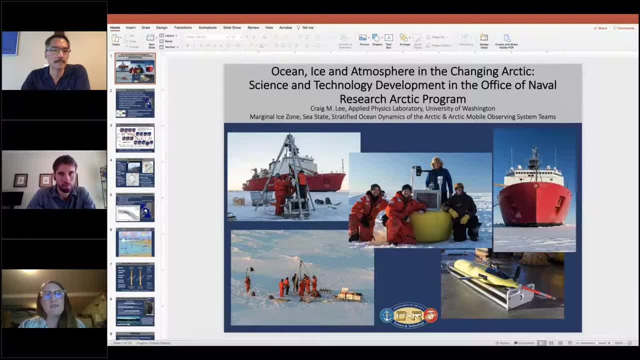 stemming from a sequence of oceanography and oceanography studies. Craig is a senior principal oceanographer of the Office of Naval Research, Supported Efforts focused on changes in atmosphere ice ocean dynamics in the Beaufort Sea. Craig is a senior principal oceanographer who leads a team of scientists and technologists that pursue 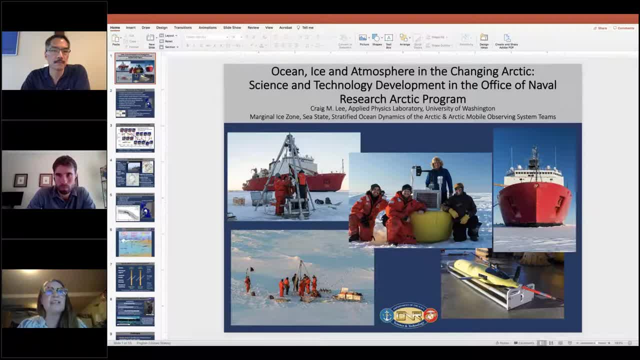 a wide range of oceanographic field programs, including intensive studies on Curriculum, Recurrent coupled physical biogeochemical studies and studies aimed at quantifying and understanding Arctic change. An important component of this work involves identifying advances that could be achieved through novel measurements and then developing new instruments to meet those needs. 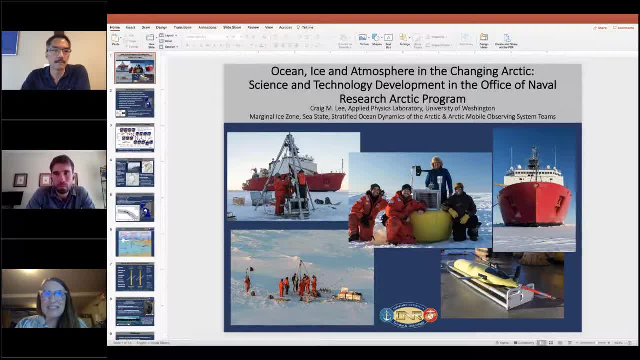 Hi, could you mute your microphone for those that just joined, please? So an important component of Craig's work involves identifying advances that could be achieved through novel measurements and then developing new instruments to meet those needs. His team's accomplishments include the manufacture of autonomous gliders capable of extended 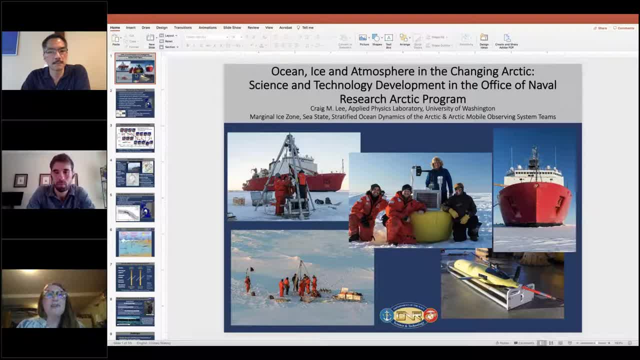 operation in ice-covered oceans. He's also a former scientist and geontologist at the US Air Force in 2018.. His research focuses on rating and I've shared a few slides with you. Craig is also a graduate of the US Department of the Australian Institute of Meteorology and Geoscience. His research focuses on the development of a new system which is called and acquired water, Including the international collaborative effort that set a new record in the survey that they did off the Antarctic ice shelf in 2018.. High performance towed vehicles and lightweight, inexpensive mooring technologies. And his primary scientific interests include upper-ocean dynamics, especially mesoscale and submesoscale fronts and eddies, interactions between biology, biogeochemistry and ocean physics, and also high-latitude oceanography. And with that I'm gonna let Craig take it away. 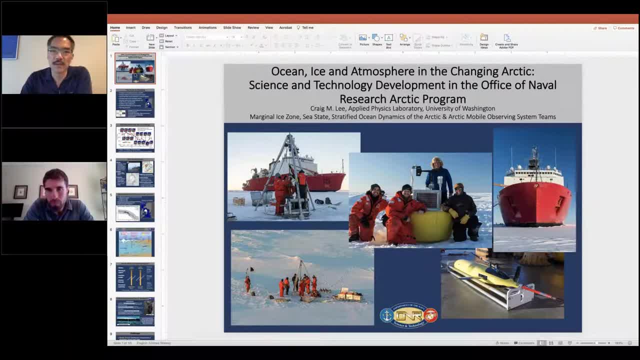 Great. Thank you, Heather, and good morning everybody. Thanks for having me here today. What I'd like to do is give you a fairly broad overview of a range of science programs that have been supported by the Office of Naval Research through the Arctic and Global Protection. 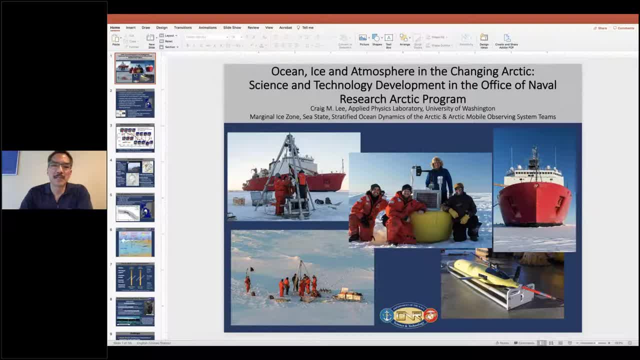 Program and things I've had the good fortune to be able to participate in. They do come together to paint a whole of those, so hopefully you'll see a common thread through these. As always for something of this scope, it's the work of many, many people in particular. 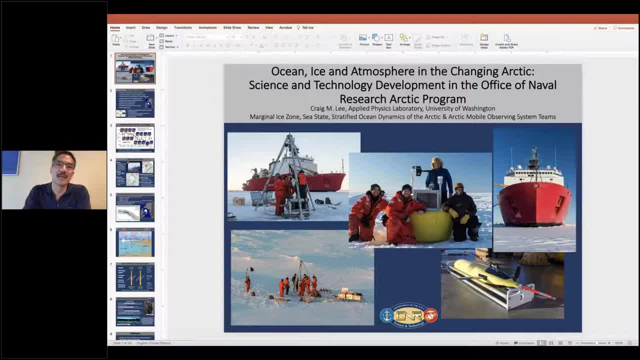 the Marginal Isis Zone, Seastate, Stratified Ocean Dynamics or SOTA team and the Arctic Mobile Observing System teams. I'll show you long lists of people, but bear in mind this is really the work of dozens of people that you're about to see. 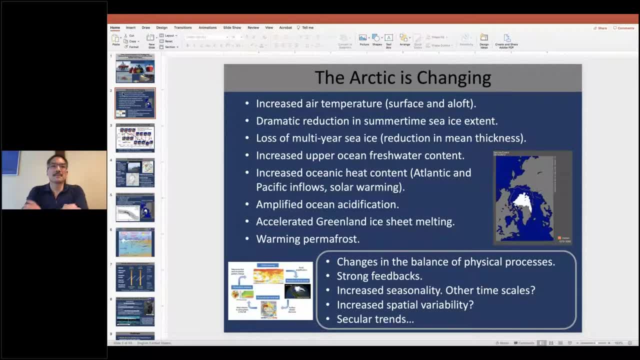 So, moving forward here, I probably don't need to explain this to this crowd, but the Arctic is really a very interesting topic. It's a very interesting topic. It's a very interesting topic. We're seeing enormous changes, which include atmospheric changes, the thing that's. 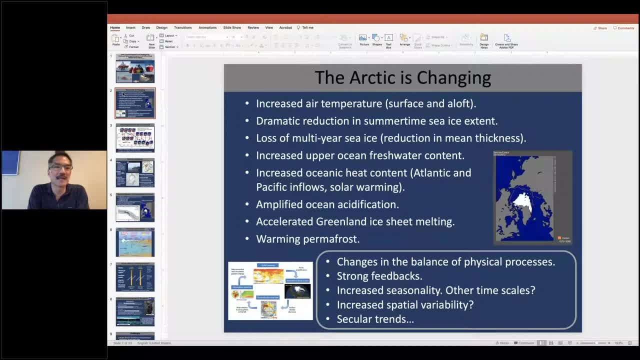 most in the news, which is the dramatic reduction in summertime sea ice extent, the loss of multi-year ice. so it's not just the extent of the ice but it's the quality and the thickness. changes in the stratification and freshwater content of the water column increased ocean. 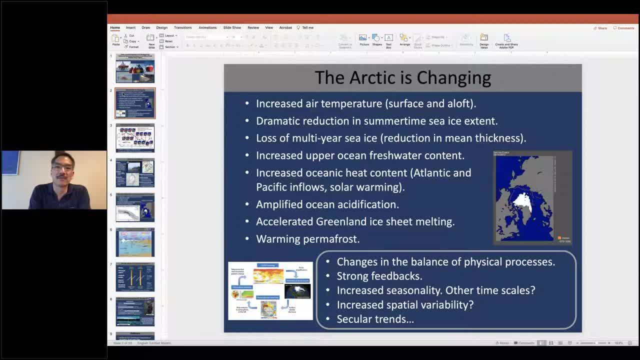 acidification, ice sheet melting, which is one of the largest drivers of uncertainty in predictions of sea level rise. So we're seeing enormous changes, which includes atmospheric changes, the thing that's most in the news, which is the dramatic reduction in summertime. 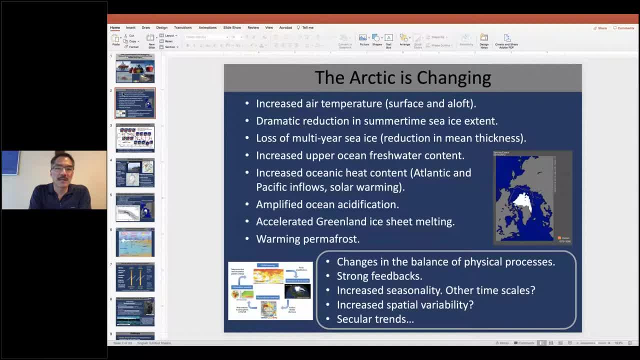 sea level rise, changes in permafrost- So all these things imply dramatic changes in the balance of physical processes that we're seeing. We think there are strong feedbacks. We're seeing increased seasonality, secular trends- so many different things that come. 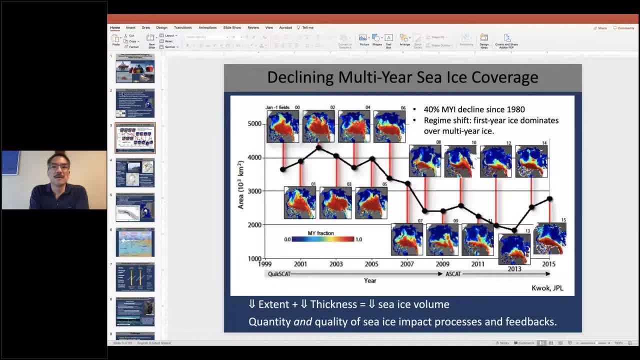 to bear in how we think about the Arctic. When we talk about changes in sea ice, which is one of our focuses, it's changes in the nature of sea ice and coverage, And what you see here from Ron Kwok. Ron Kwok is a plot that shows you a change in the aerial coverage in multi-year sea ice. 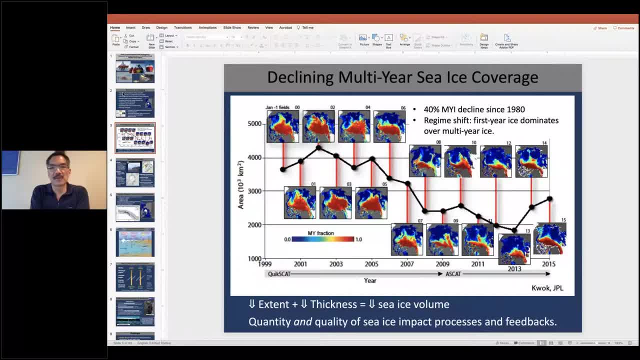 So the dark colors are significant fractions of multi-year sea ice. The light colors are either open water or first-year sea ice, and it goes from 1999 to 2015,. so not even the most recent measurements. But what you see is what used to be large extents of multi-year 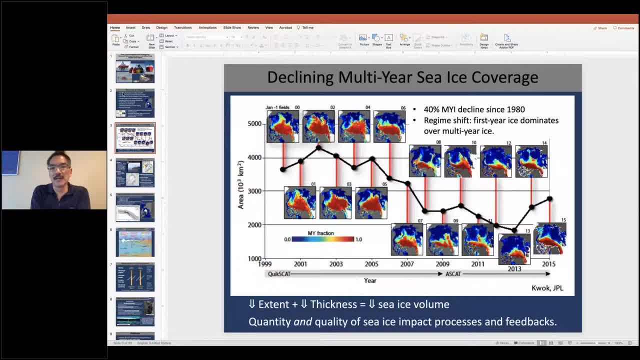 sea. ice clustered near the Canadian…in the Canadian Arctic has now become a thin band North of the Canadian archipelago in Greenland and the rest of it is really really fairly thin first-year ice And this means it's more mobile, it's weaker. We have many, many 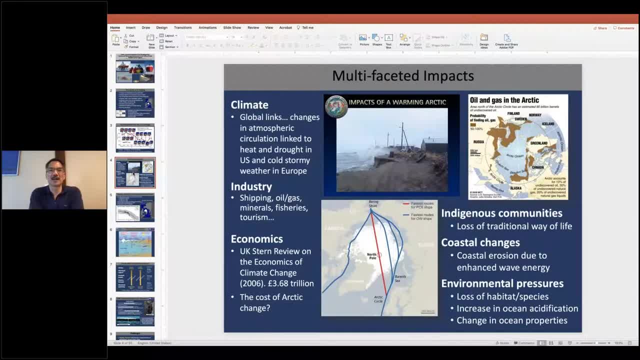 different changes in ice quality that change the dynamics. So these changes have huge impacts. Of course, there are climate changes which have impacts, which have really global ramifications. We could go on at length about the connections between Arctic and middle altitude climate. There are impacts to the local communities. 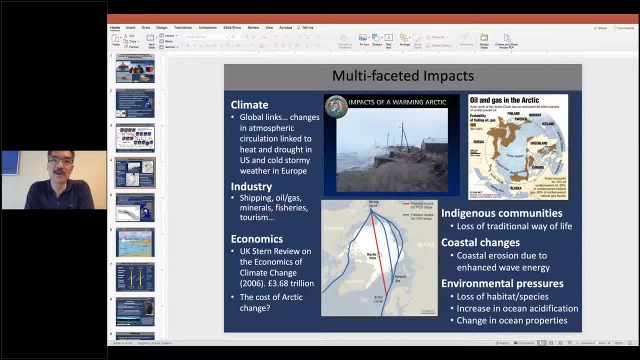 and the center picture. there you see increased surface wave activity eroding the shoreline in one of the northern communities in Alaska. You see increased opportunity for shipping for oil and gas exploration right for resource extraction in general. So lots of different possible changes that have implications in terms of what we need to know to plan those. 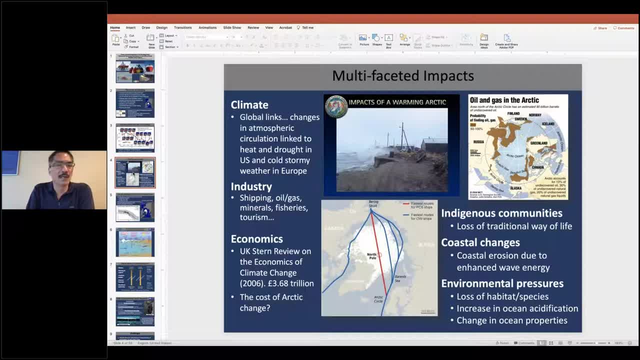 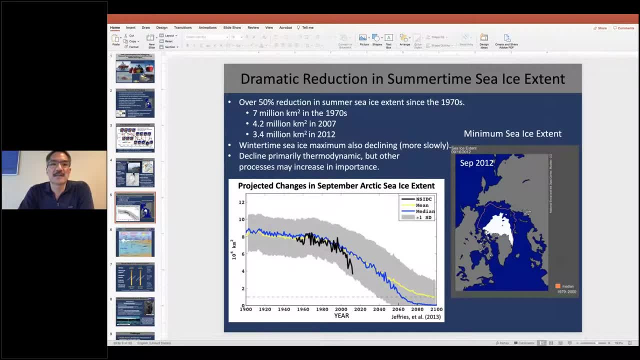 changes to plan activity And what we might need to know to respond to emergencies. If we come back to the reduction in sea ice extent, one of the interesting things to us- and this is what…one of the things- that motivated the Marginal Ice Zone experiment. 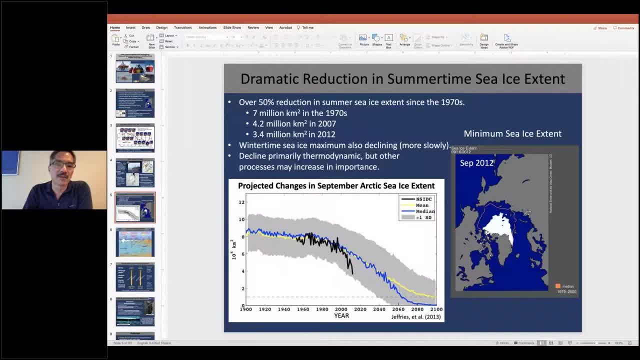 which we'll talk about in a minute, was looking at both the observed and the projected changes in summertime sea ice extent, where, if you look at the plot in the bottom left-hand corner you see the mean and the median of the model results. 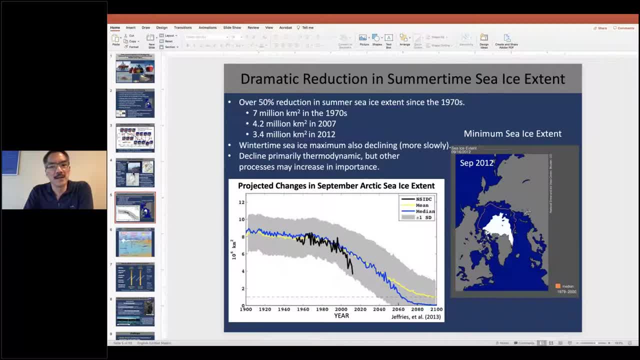 And then you see the observed sea ice extent changes in the black, And what you see is that the observed changes in summertime sea ice extent are barely within the one standard deviation range of the model results. A couple of years prior to this, it wasn't…the observations. 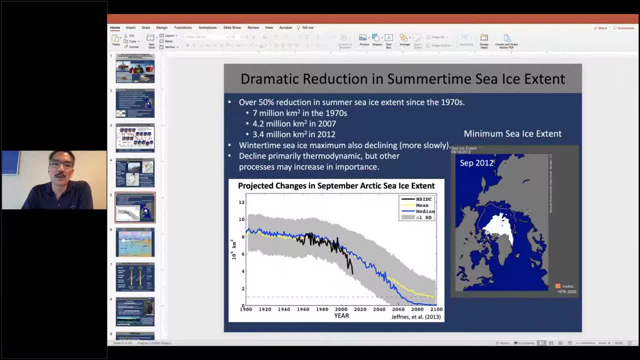 weren't even really within the range of the model predictions. So what we're seeing is that the…if we just think about summertime sea ice extent. right, those changes are happening more rapidly than what the models are predicting, And what that tells us is that we don't really completely understand the physics that are. 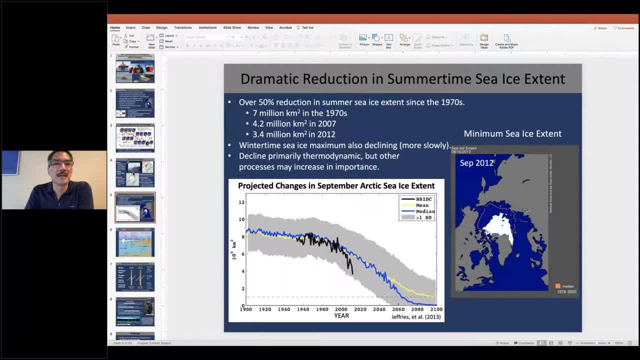 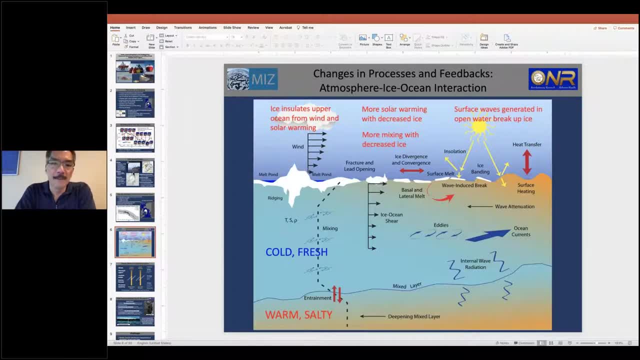 driving that decline. So ONR has invested a fair amount of resources in trying to improve our understanding of the physics. You know, any good process study starts with a cartoon, right, And so this was the cartoon that drove the Marginal Ice Zone experiment And really what we tried. 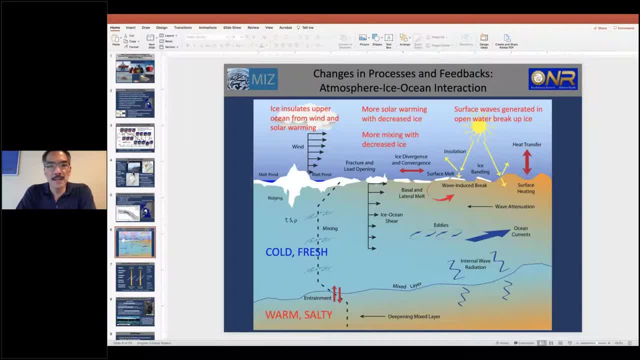 to portray here, if you go from left to right, is that the conditions under full ice cover right- the old Arctic and then increasing…the increasing…increase and decrease in ice cover right. increasing amount of open water as you move into the new Arctic. So in the 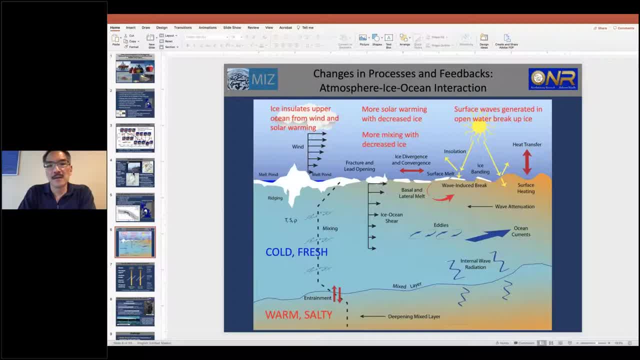 old Arctic. the ice isolated the ocean from atmospheric forcing. The Arctic is, of course, this upside-down ocean, where you have a cold, fresh halocline that isolates warmer, saltier layers below, And those warmer, saltier layers could be a near-surface temperature maximum. 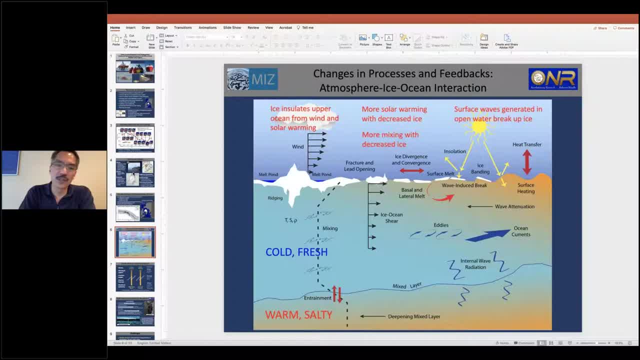 formed from the summertime impact, And so let me just go through the data—so we've got the Arctic Ocean, We've got ice layer out and that's the Arctic Ocean of the Arctic Ocean. right So the Arctic Ocean. 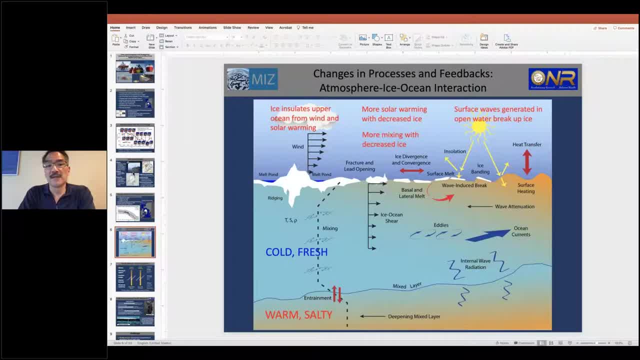 is one of the major points that's going to be removed from the Arctic Ocean, And so that's basically be done under the 혼자 later winter time. That's probably what things like fire are going to be, so that the Arctic Ocean is going to be, you know. 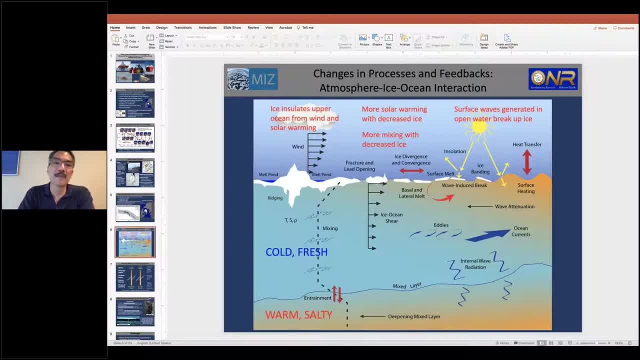 all of the Arctic Ocean. So basically, you know, the Arctic Ocean is going to completely split the Arctic Ocean into distinct parts. Yeah, so the Arctic Ocean is going to be constructed from polar-solid and the Arctic Ocean is going to be completely separated from the Arctic. 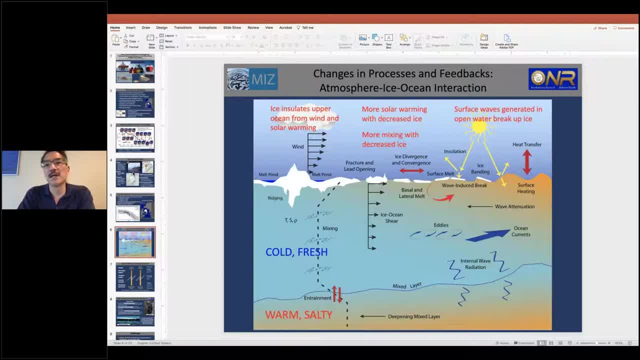 both from solar radiation and from momentum input, which would generate internal waves at ease, mixing right. But as you see increasing amounts of open water, as the ice gets weaker and you get an increasing open water fraction, the ice gets more mobile, It gets more efficient in momentum transfer. 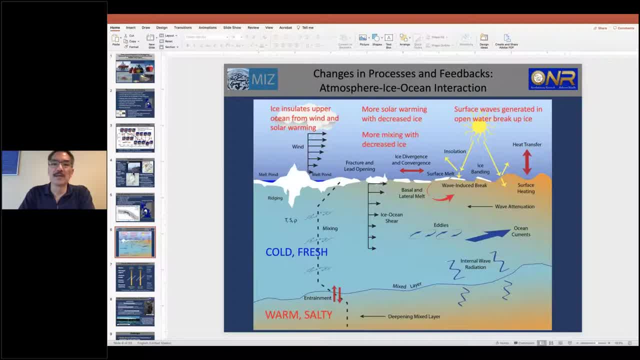 between the atmosphere and the ocean, And so you suddenly have the ability to input momentum, generate internal waves, generate up-ocean mixing at rates that are perhaps more efficient than they would be in open water, And so you see mixing and therefore an ability. 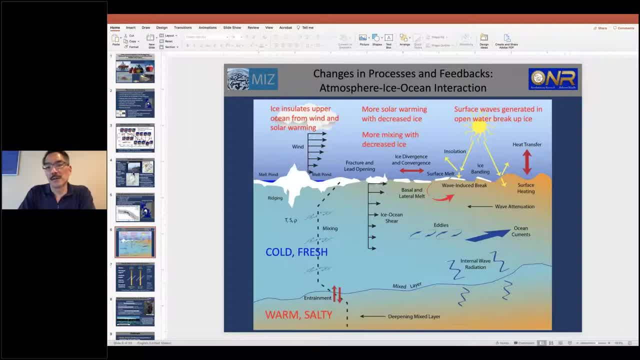 to bring that heat up from the layers below And then, as you get lots of open water, you get the ability to generate surface waves, And those surface waves- you get increasing amounts of fetch and more wind activity- have the ability to propagate into the ice pack. 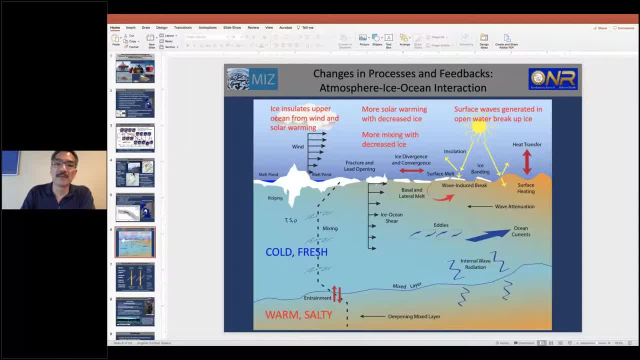 and do mechanical breakup of the ice right. So that was one of the thoughts was that perhaps the increase in surface wave activity would be driving increased mechanical breakup of the ice, And so you can see some of these are positive feedbacks, right. more open water, more surface waves. 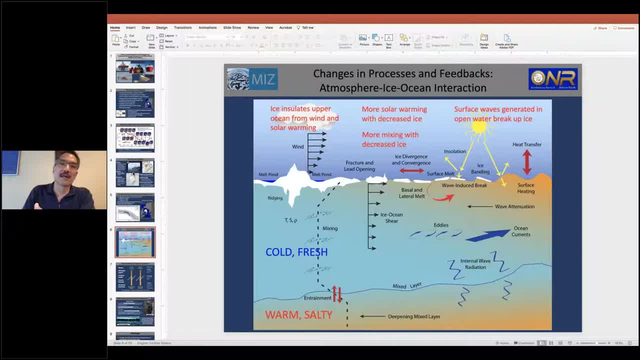 more mechanical breakup, more open water. There's the famous ice albedo feedback, where you get more open water, which is dark, you absorb more solar radiation, which generates more melting. But there are also negative feedbacks that, as the ice melts, 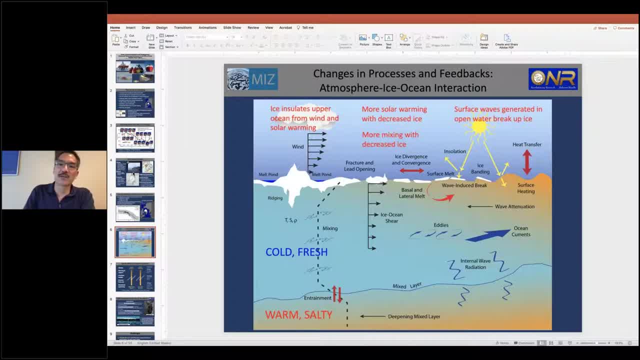 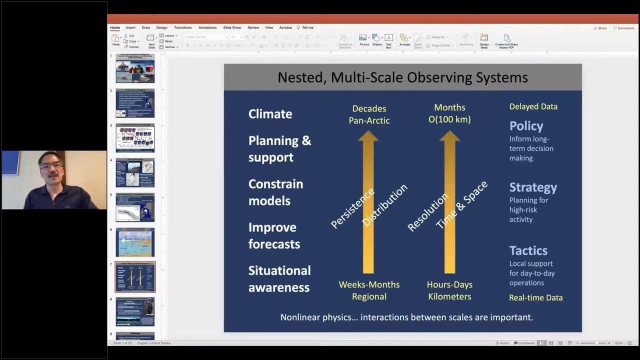 you inject fresh water into the upper ocean, which is stratifying, which therefore isolates the lower layers from mixing. So part of the game is understanding how those- what balance of feedbacks plays out in the New Arctic. In order to understand these things, 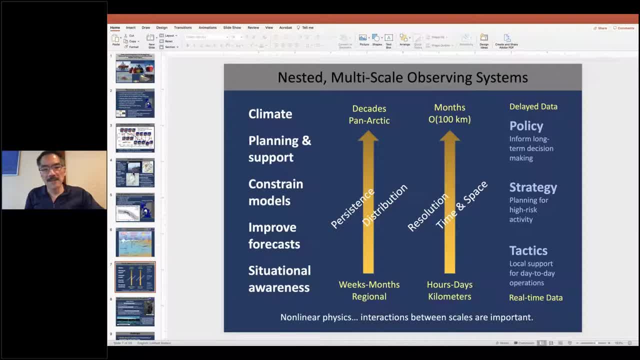 we think about a need for a nest observing system. I tend to use this diagram to indicate the difference between- right, if you look on the left-hand column- the difference between measurements that we use to understand climate, which are very long-term and distributed. 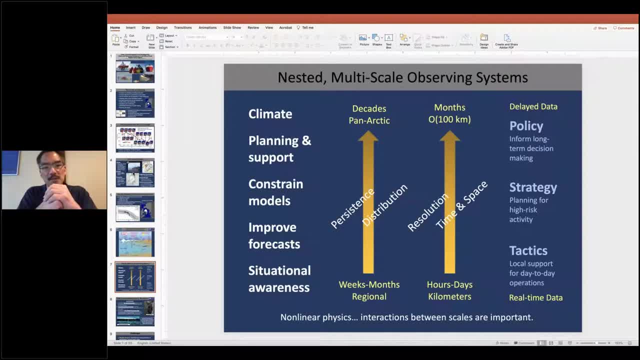 as you move down that column, the measurements we need for situational awareness, which are very, very limited shelf-life. You need the measurements right away, but typically you only need them in a very limited area right to understand what's going on. 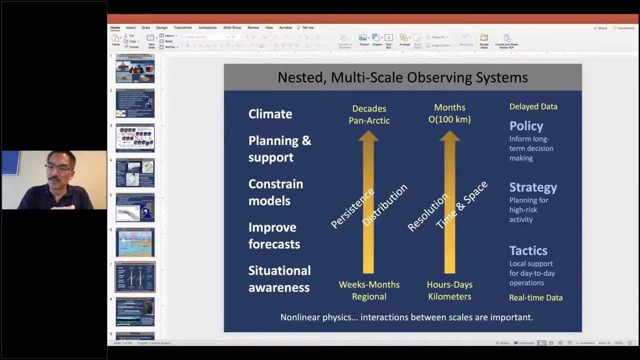 And everything in between. which measurements used to constrain models right, Maybe a little broader, maybe a little more timely delivery. You can think about those in terms of policy and decision-making right. Long-term measurements, Strategy- what do I need to do next year? 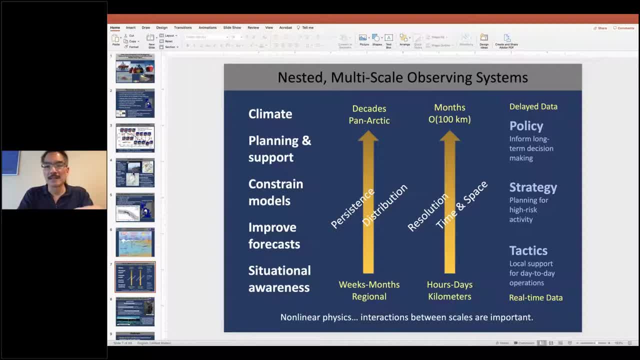 or the following year. The ability to make those final decisions. forecasts and tactics. support for day-to-day activity, ranging from is it safe to navigate a ship through the ice here to if I'm a hunter, can I go out on the ice today? 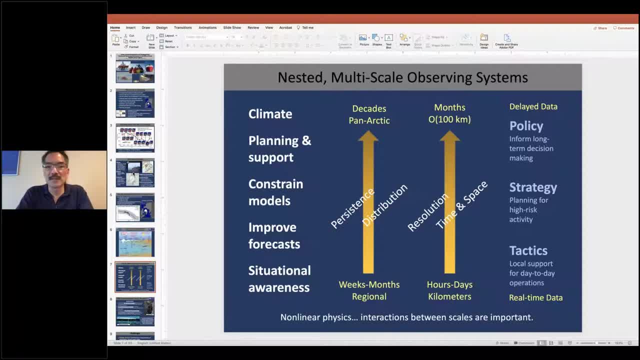 Right. so these imply different time scales and different spatial scales of those observations, Range of them distributed pan-arctic to focused regional observations, and observations of resolved scales, of just seasons or months to really observations needed at hourly time scales. And the problem here is that the physics are non-linear. 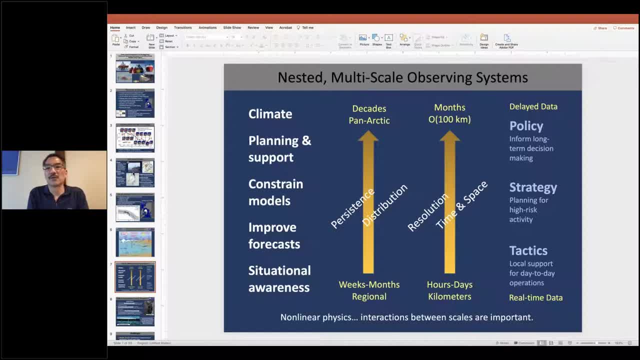 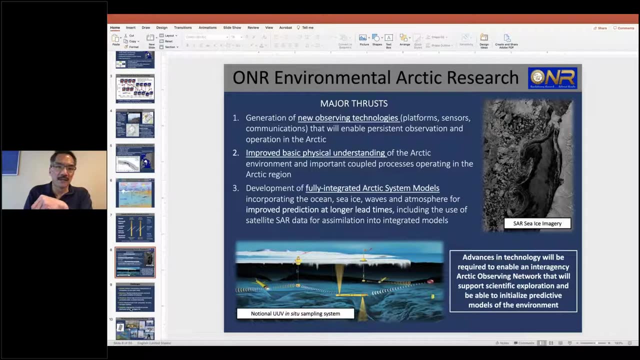 So the interactions between the scales are important and in order to really make predictions at some of these timescales you need to understand the dynamics at shorter timescales and shorter spatial scales. So there kind of is no shortcut. ONR has been interested in a variety of these things. 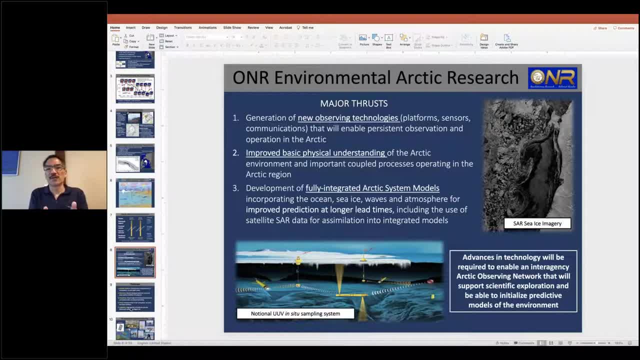 and to make this short, ONR has been very interested in developing technologies to make these measurements and improve physical understanding. So, process level, understanding of the dynamics and then all feeding fully integrated arctic system models right. So that's been the thrust within the ONR Arctic. 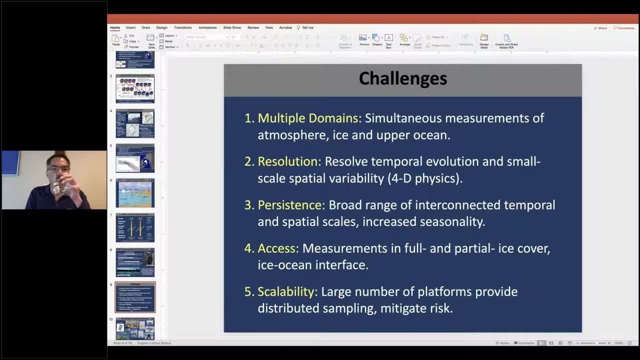 and Global Prediction Program and why those two sit under the same program. The challenges, of course, are that we're trying to observe over multiple domains- atmosphere, ice and upper ocean- which are not easy to observe at the same time in the same place. 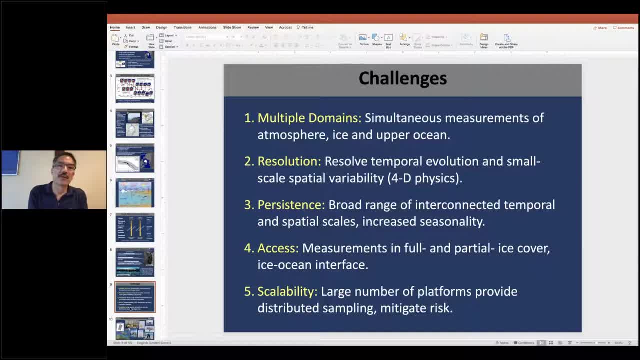 Need to resolve at a variety of scales. The physics are fundamentally four-dimensional. We would like to have persistence, the ability to stay up there over a long period of time, So we understand those interconnected scales. Access is difficult, right Making measurements under the ice. 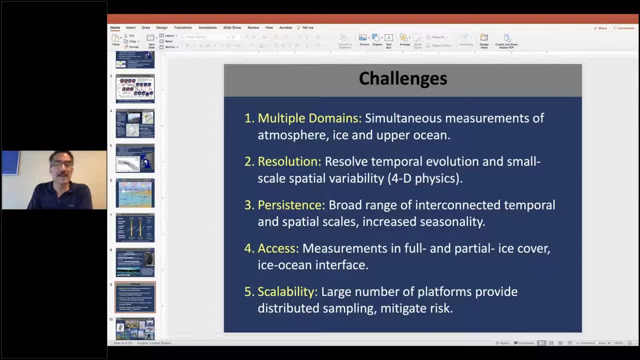 is particularly difficult- those scales- Then we'd like to be able to do that in a way that lets you range from focusing on a small area to making more broader, distributed measurements, So something that's highly scalable. We're fortunate to live in a 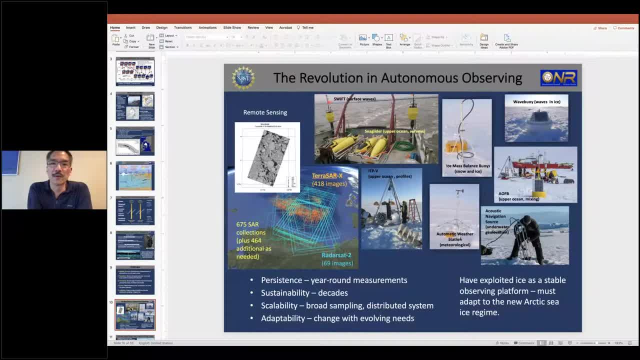 a time when, when robotic measurements are becoming widespread, right, Our ability to make measurements with small rental, relatively inexpensive robots is exploding. And I'll talk about a variety of these platforms. I won't go over them in detail here, but fundamentally, when you combine these robotic measurements, 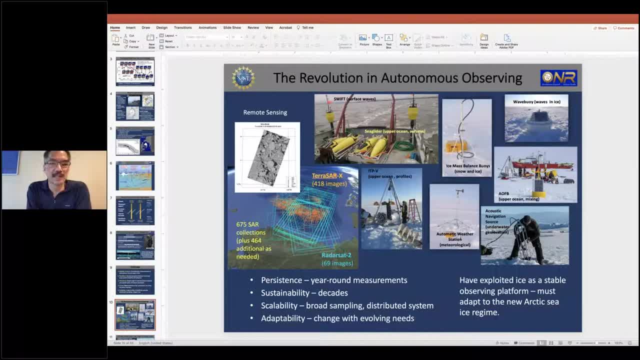 with some more conventional measurements and the ability to collect widespread remote sensing, we can now achieve that kind of persistence and sustainability that we've been after for such a long period of time. We're getting to a point where we can- you know, we can- scale the measurements over broader areas. 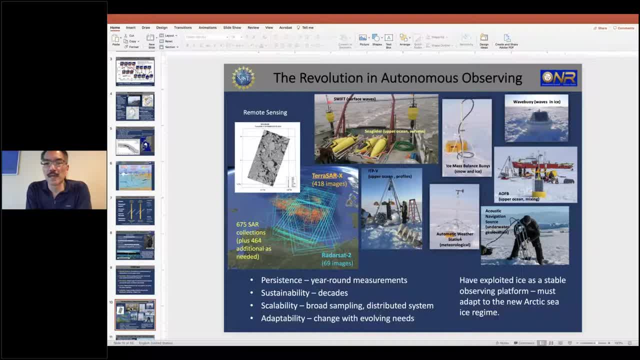 And I think we're also getting to the point where we're able to make more adaptive measurements. One of the keys of this has been to use the ice as an observing platform. right, It's a nice, stable observing platform. we can put things on. 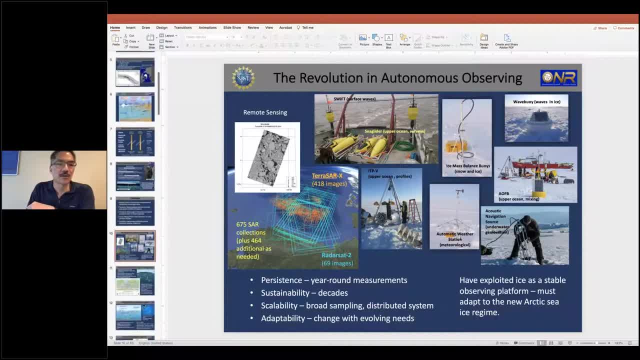 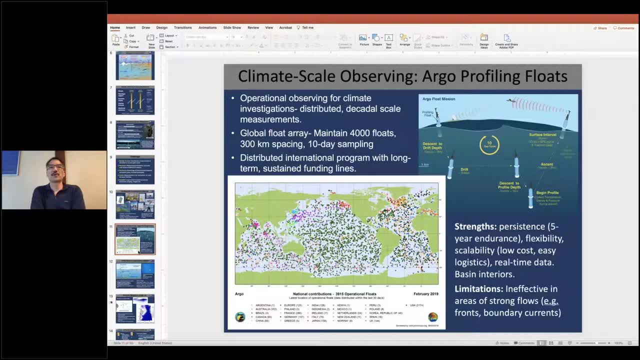 That's changing as the Arctic changes. It's getting harder and harder to use the ice that way, Harder to land on it, harder to put instruments out there. We'll be out there for a long period of time. So right, any talk about robotic observing. 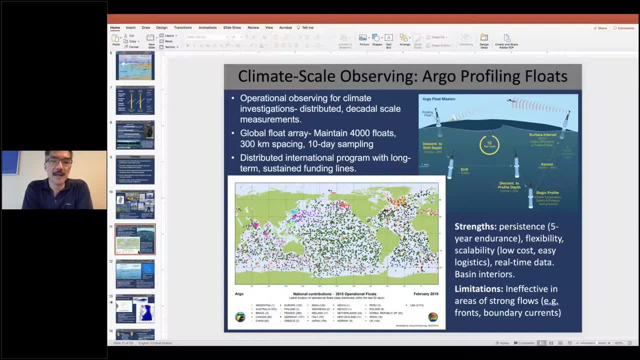 has to start with floats. They've really been the game changer in how we think about observations in the ocean interior. They're operational for physical floats and becoming operational for biogeochemical floats within the global ocean. These are still harder for the Arctic right. 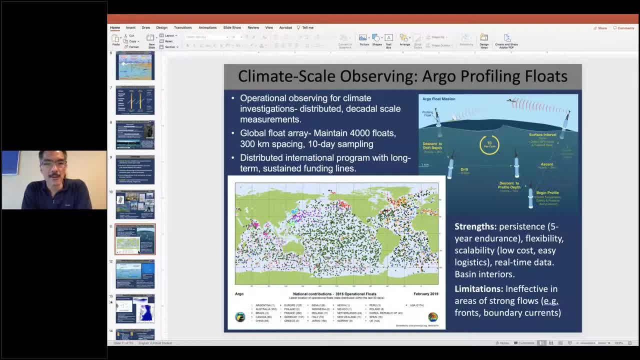 We can do five-year deployments of floats right now, one profile every 10 days with a network distributed over an entire ocean. But in the Arctic we've been able to do a lot more than that. Geolocation is still difficult. Data exfiltration is difficult. 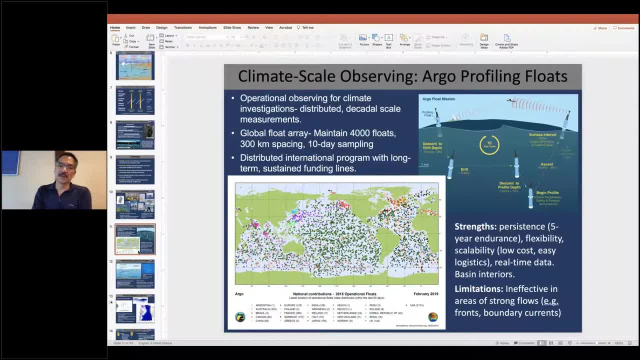 because you need to have satellite service to get the data out. So float deployments in the Arctic are still in their infancy, but they are still. they are happening and always been one of the leaders in doing that, The platform that I've been most involved in developing. 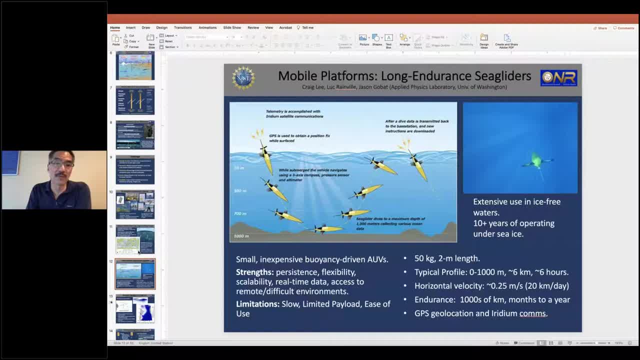 with my team, is the lead developer for one of the three glider production glider platforms for sea glider. These are small, inexpensive, buoyancy-driven vehicles. I won't belabor this because people are probably aware of them Being 50 kilograms, two meters in length. 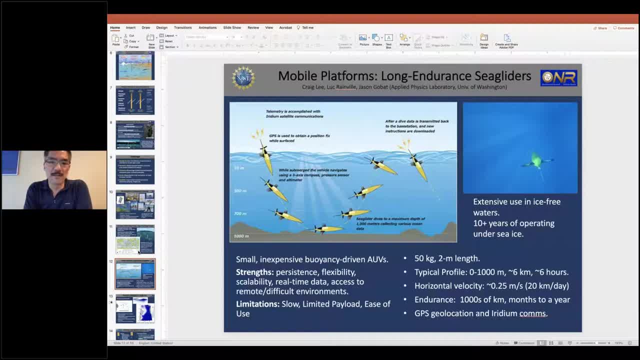 pretty routine year-long operations in ice-free waters now And we've been learning to operate them in ice-covered waters, but we've been doing that for about a decade And we've achieved year-long deployments in Arctic sea ice and in Antarctic sea ice and ice shelf environments. 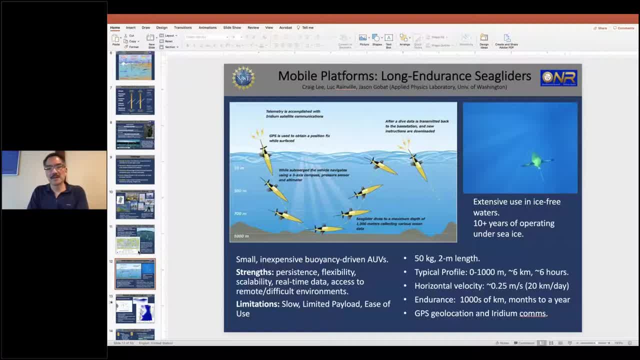 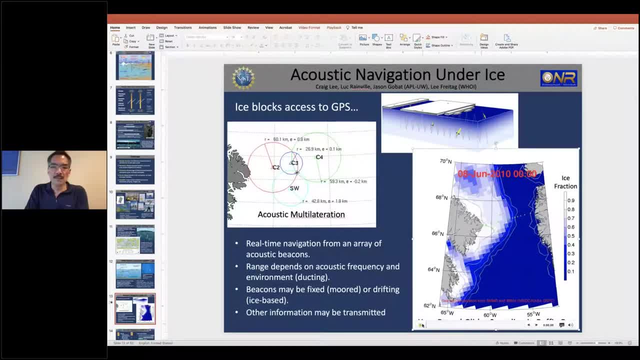 we need to be able to navigate under sea ice, And we do that by in the dumbest way possible, really, which is by multilateration: putting out beacons where you know the location of the beacon, The beacons broadcast on a known schedule. 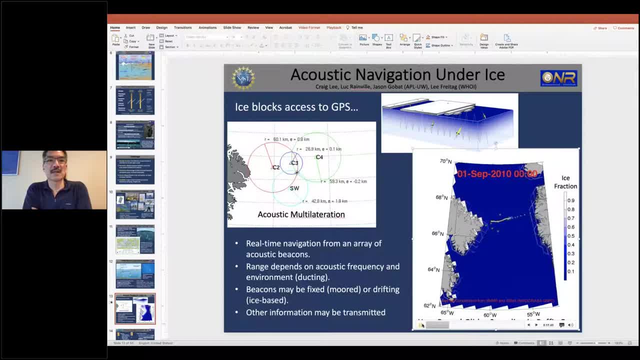 When a vehicle hears those broadcasts, it can calculate, it can say a range and you get multiple ranges. you can draw rain circles and look at the intersection between those rain circles to to achieve a position estimate. and what you see in the animation right now that's going is the other deployments in davis strait, which are really our first. 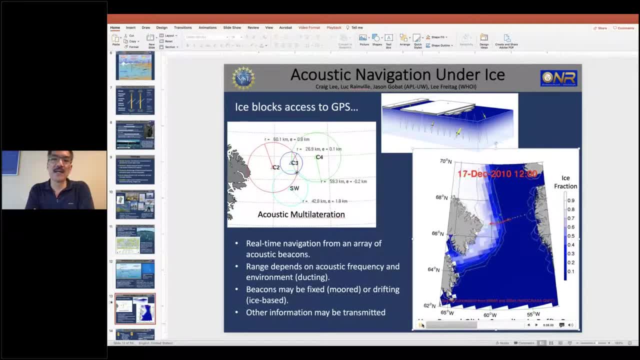 deployments of the ice and you see glider marking back and forth across the strait. the ice is coming in white right now. the blue is open water and what you'll be able to see is the glider navigating back and forth under the ice. now it might be difficult to see in this display. 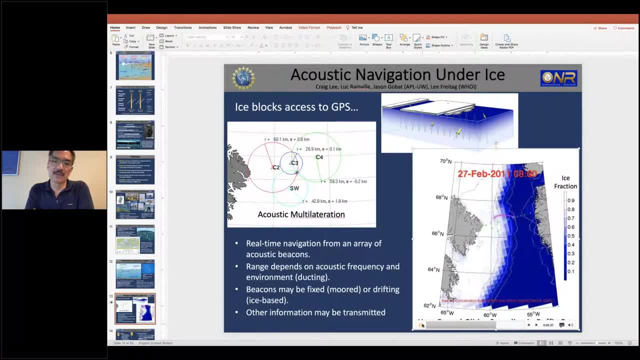 but there are a number of circled moorings, green dots, which are sound sources, which is what the glider is navigating from. fixed location navigation gets rougher as the glider starts to go under the ice and that's because we go from navigation which has meter accuracy. 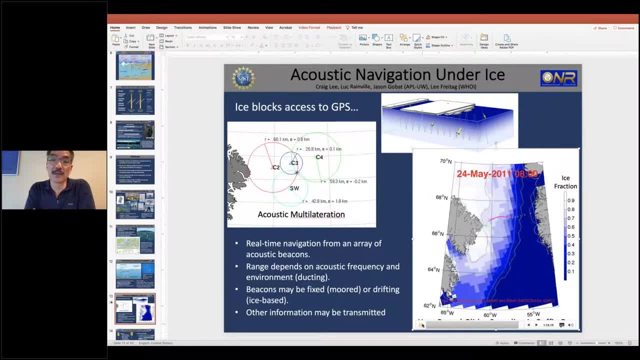 to navigation that has roughly kilometer accuracy. we can no longer calculate depth average currents, so the glider gets pushed around at the currents more. but that gives you an idea of a year-long deployment of operating under the ice in the strait. as i said, those, those measurements are roughly 10 years old now, those operations. but 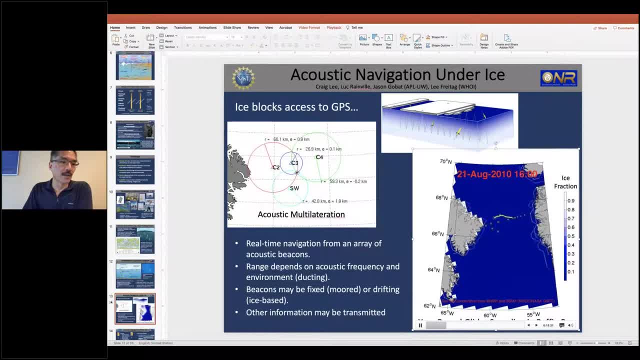 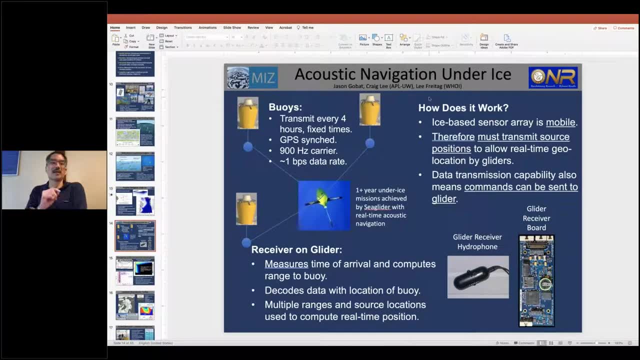 that was really the first, the first go at doing that. so how that works. again, the modern system uses 900 hertz broadband sources from the fry topic. the sources transmit every four hours. they can, because they're broadband, they can transmit some information on the signal we choose to. 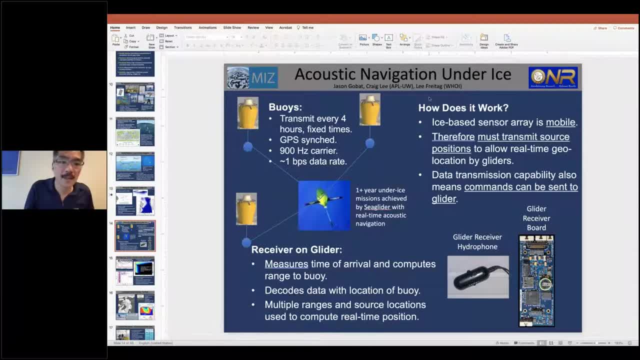 transmit the location of the source or the location of the transmission. so now the sources can move, they can be more than on the ice and they can drift and the glider or float can navigate from those. this also allows us to send a very limited command set to gliders and floats, say: 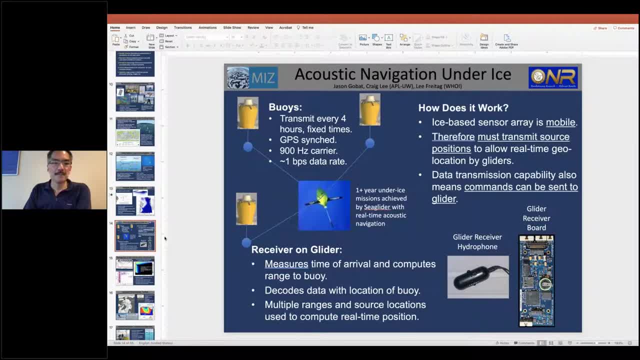 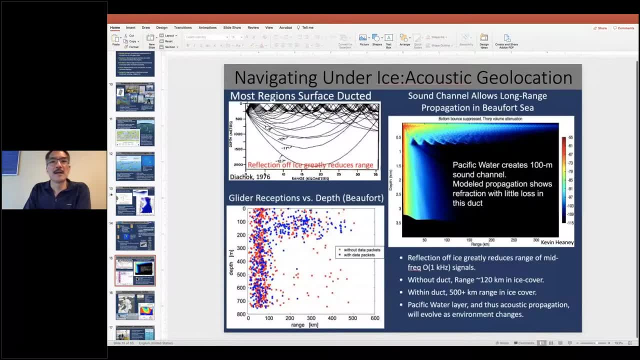 commanding them to adopt a new sampling pattern, or commanding floats if you surface more frequently to uh to try to collect positions or report data. one of the interesting things about the beaufort, about the western arctic, is it now has a sound channel. the pacific summer water comes in, provides a sound channel of roughly 100 meters, which gives us 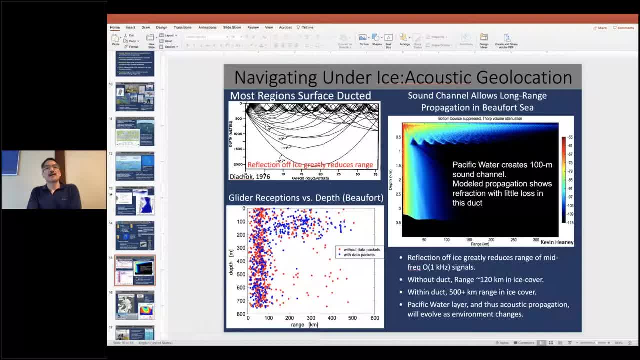 roughly 500 meter range from the sources. sources are transmitting and most of the arctic have only about 100 meter range because they're surface adapted, meaning that the transmission reflect off the ice bottom, which is pretty lossy, and they don't go very far. a demonstration of 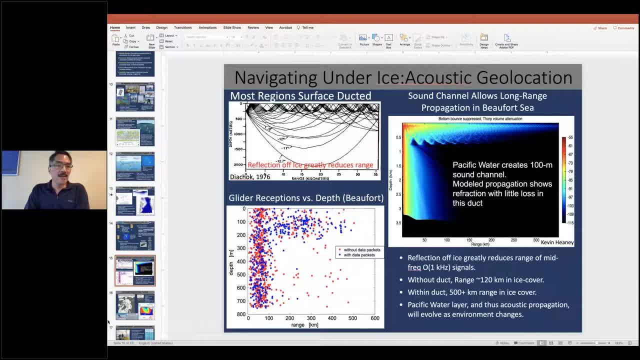 that if you look at the uh, if you look at the bottom left here for transmissions in the beaufort uh, you can ignore the red and green dots. they just have to do with whether or not the data packet was decipherable. but what you see is that in the uh, in the sound channel, at 100, meters, we get ranges out to 500 kilometers outside of the sound channel. right deeper we get ranges all the way out to 100, 150 kilometers, which would be more typical of the general arctic. so that pacific layer might change over time. um, you fully might expect that it would change as the arctic changes. 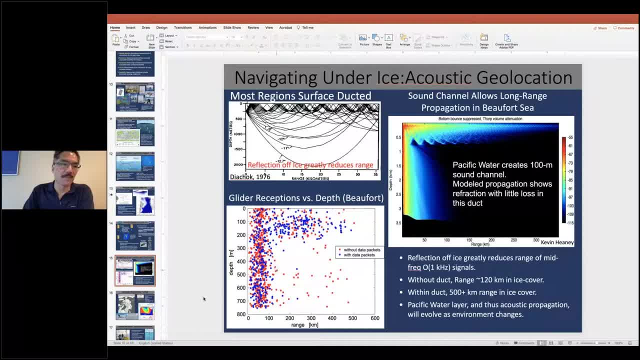 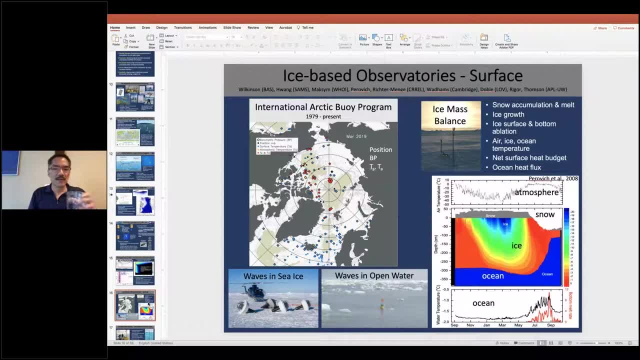 and as that changes we may lose the sound channel and go to a a more general arctic sound channel which has fairly limited ranges. so the other other platforms we depend on in the arctic are ice based. um the international arctic buoy program, that's been going since 1979, so it really is the oldest operational. 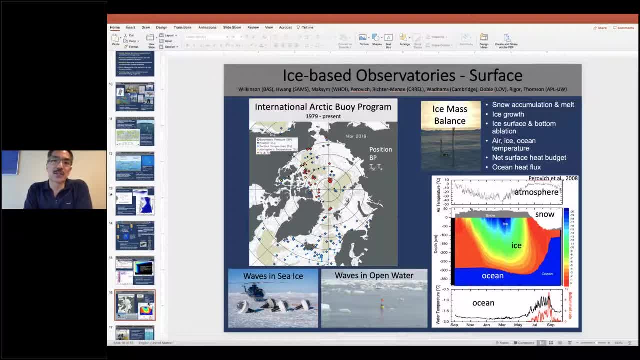 observing system in the arctic. it measures just position and barometric pressure and air temperature really on the surface. we also use ice mass balance buoys that tell us something about the structure and nature of the ice as it melts out and have the snow on top of it. 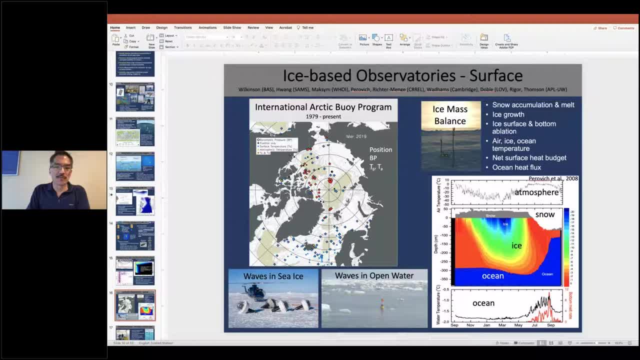 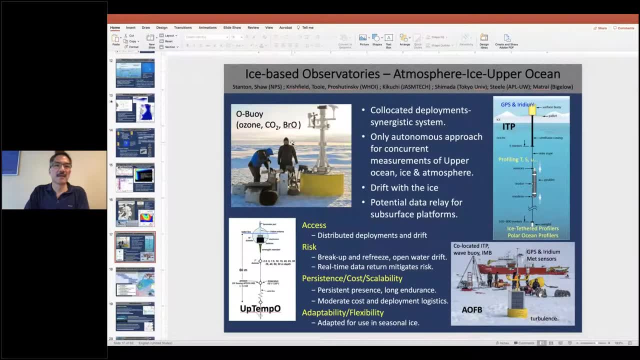 and surface buoys, either on the ice or in the open water, for measuring surface waves in the ice extending to the water column. they're instruments like the, the ice tether profile, which has had great success measuring measuring profiles on the ice from an instrument mounted on top of the ice adrifts arctic ocean flux buoys, which are 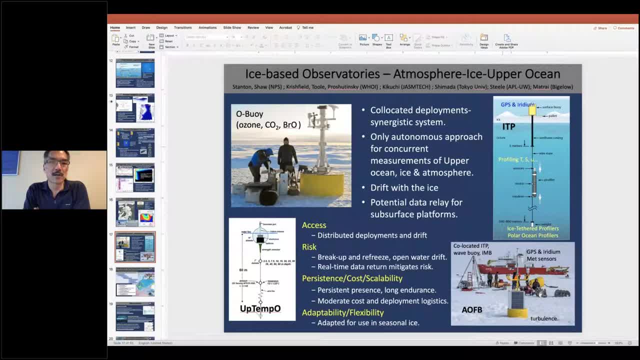 really aimed at measuring turbulence in the upper part of the water column, the old buoy which measures chemical properties and then operation temperature buoys- so you know a zero different blue- that are mounted on the ice and make measurements down below. So ONR has funded a range of research programs. This gives you an idea of 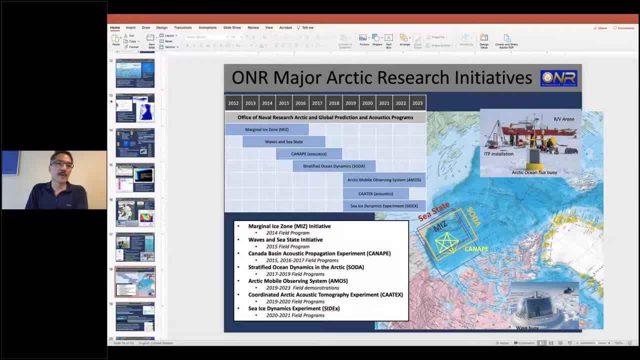 those programs plotted out over the years. We're going to focus on the Marginalized Zone Program and the Stratified Ocean Dynamics Program, with a mention of Seastate here, but you can see that there have been others in between. They all focus in this area of the central Beaufort. 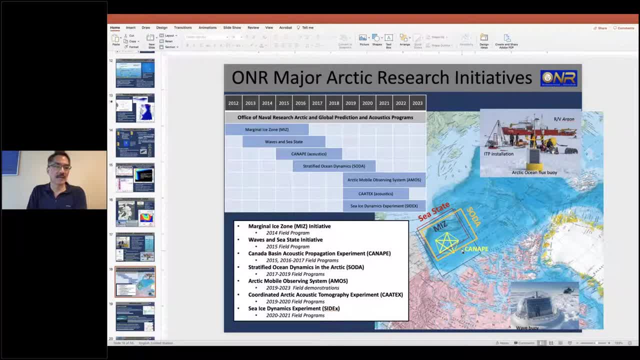 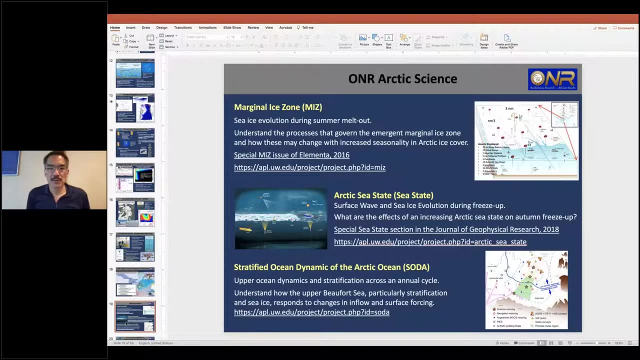 in one form or another. so that really has been the focus of that sequence of research efforts. Each of those efforts is roughly five years long, typically with a year of intensive field measurements. So to give you some contrast between three of those programs, Marginalized Zone was 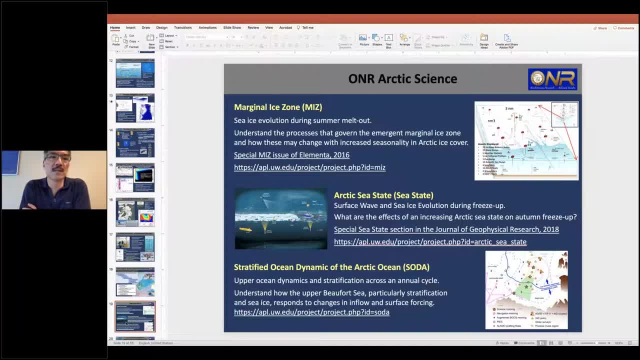 focused on the springtime meltout, spring and summertime meltout. It was really focused on that interface between the, the open water and the pack, so that area of broken ice that's hard to make measurements in, because instruments mounted on the ice get ejected at that point and die, whereas the open water 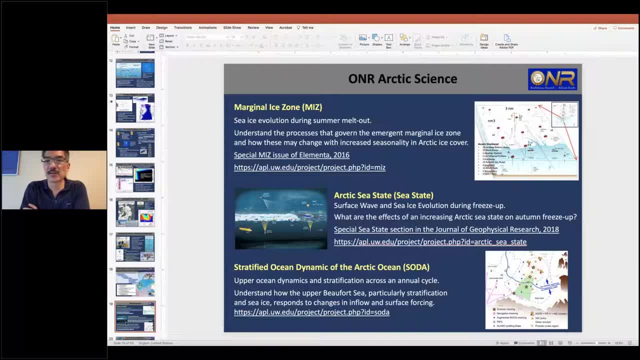 instruments that were more typically used don't have access to that region fully, But the idea was to try to understand the changes in dynamics as you walk back away from the Marginalized Zone and how that impacted the melt. The Arctic Seastate Program looked at freeze up and 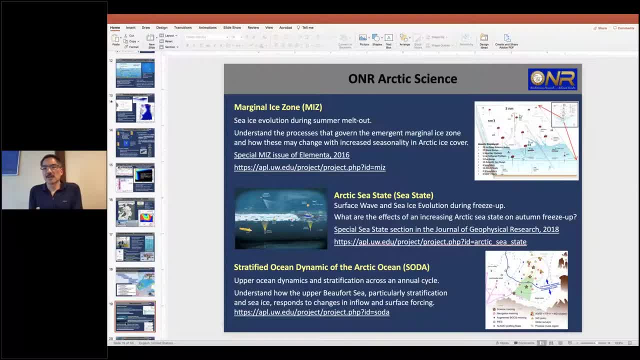 was really, really focused on that period in October, November, when the ice was coming back in and trying to understand the impact of sea state or increasing wave activity on that freeze up. So two programs focused on the ice and then the Stratified Ocean Dynamics of the Arctic Program. 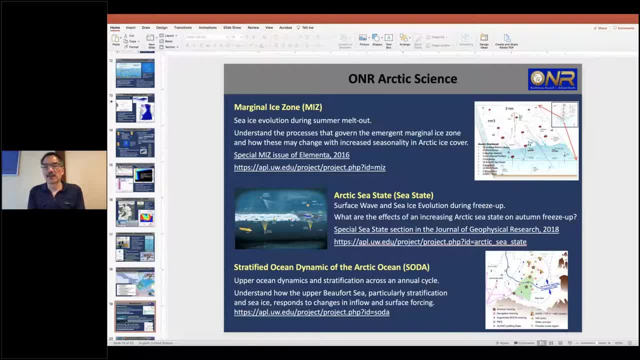 SOTA really was focused on the operation dynamics. so looking at the upper water column and how that was evolving during the the during the period of time. So, as you can imagine, the Marginalized Zone Program wanted to work in an ice-centric frame. The other two programs were 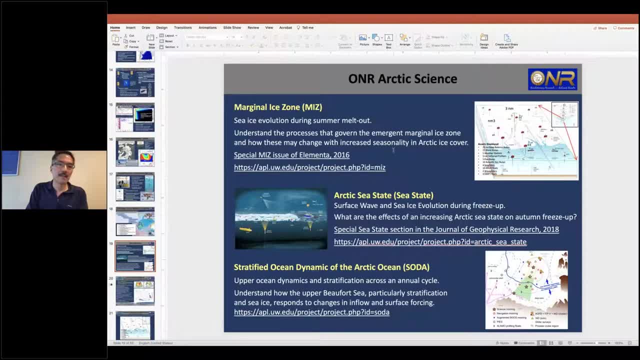 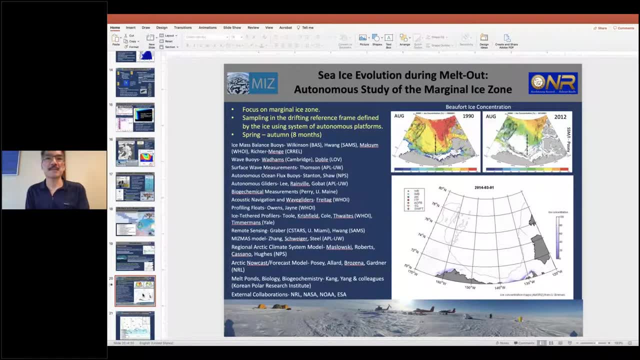 a mix of Eulerian and Lagrangian measurements. So we'll go to the Marginalized Zone Program, Again focusing on the Marginalized Zone, Because we were doing that. we wanted to focus on a drifting reference frame moving with the ice. I'll start the animation here so you can see that. 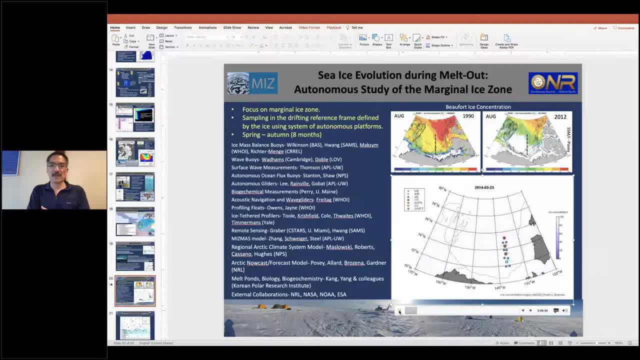 We're doing the editing view here because we couldn't quite get the presenter of you to work on the GoToMeeting. So what you see here: we deployed a carpet of instruments using aircraft very, very lightweight, so just a couple of twin otters and a Bell 212, a Bell 412, pulling these. 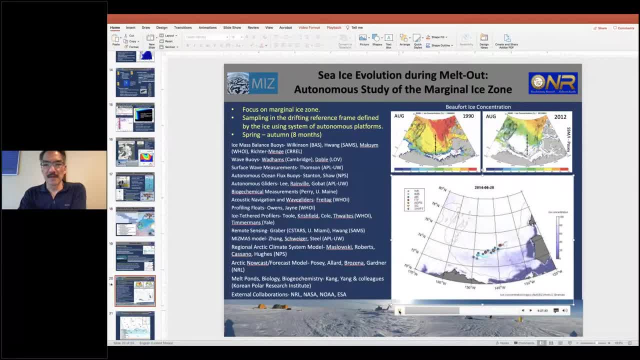 out on the ice early in the season. The idea was to have this carpet so that it would melt out and you would see this contrast between things at the Marginalized Zone and going back into the pack. But the ice was more mobile than it had been in the past and the drift pattern was different. 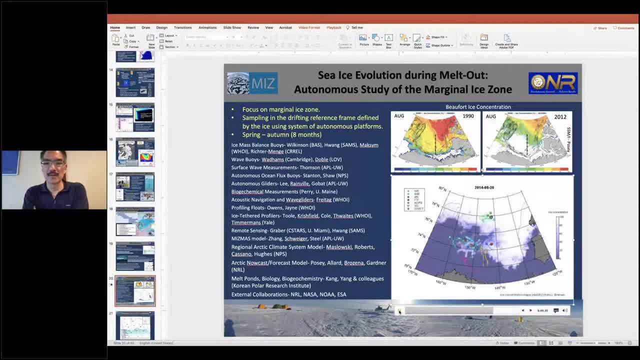 so we really ended up with things strung out. You see in yellow sea gliders being deployed and moving into the ice, right, So they're actually sampling the Marginalized Zone into the pack and back up to open water and then everybody's running away as that forms again. 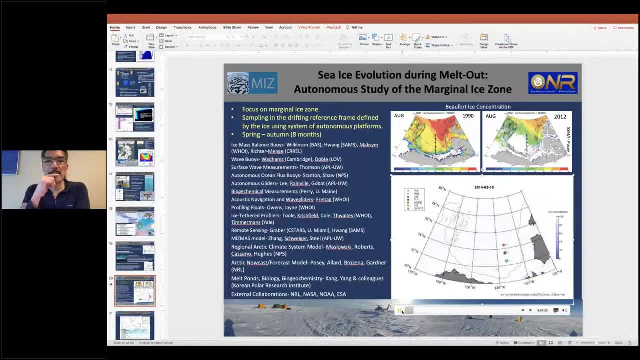 I will play that. It's going to loop again as we talk here, But really this was motivated by the fact that the Marginalized Zone plays an increasing role in the New Arctic. It used to not be much of a Seasonalized Zone and the Marginalized Zone was 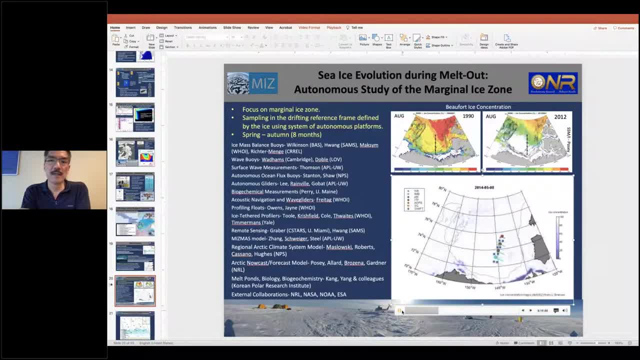 fairly small relative to more modern times, when the Seasonalized Zone is huge, occupies an enormous part of the Beaufort and the Marginalized Zone is a big part of the program, a big part of which you see in environmental variability And you see this very large list of collaborators that 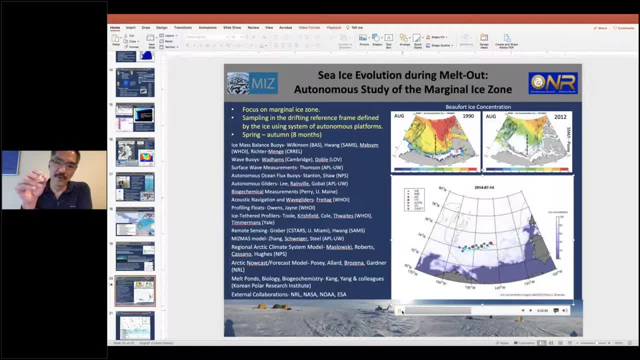 was required to make this all happen, where different people focused on the Marginalized Zone, Those of us who were focused on the ice, those of us focused on the upper ocean, remote sensing and colleagues at the Korean Polar Institute. So what I'd like to do next? I'll just show you a cartoon of how that Observing System looks. 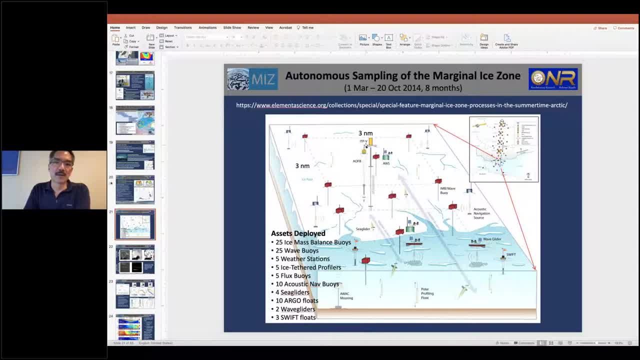 So this is one of the smaller arrays right where we put out an array of wave buoys and an array of profiling instruments looking at the upper ocean and the ocean, the sea ice, and then had gliders moving back and forth between the open water back into the pack. 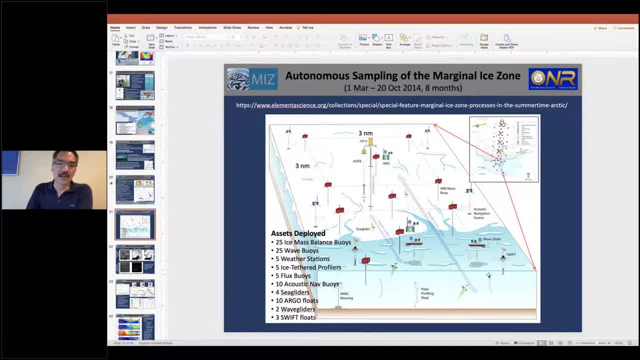 and through the marginalized zone and then wave gliders and other instruments looking at the open water on the outside, but roughly 100 assets deployed in this carpet, again with the idea that you'd have open water measurements, measurements at the marginalized zone, with these instruments being kicked out as they melted out and then maintaining an array of instruments. 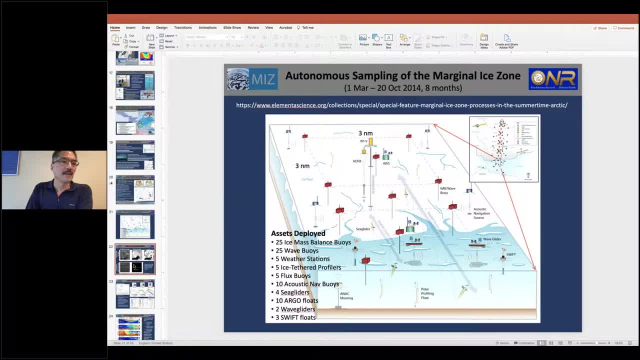 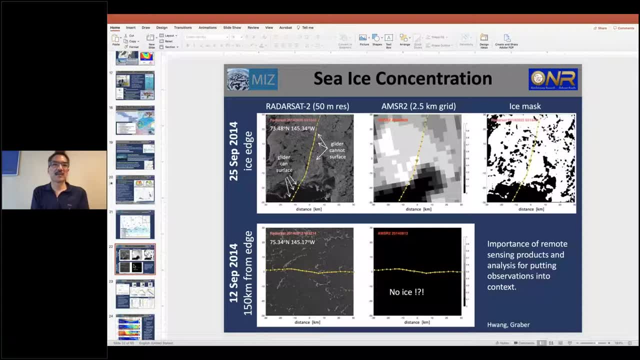 moving back with the pack, all bound together by remote sensing. so this gives you an example of the kinds of things that we were doing with remote sensing, where you would try to use it for for navigation and access, but then also create sea ice mass and flow size distribution charts that we could use during the analysis phase of the program. 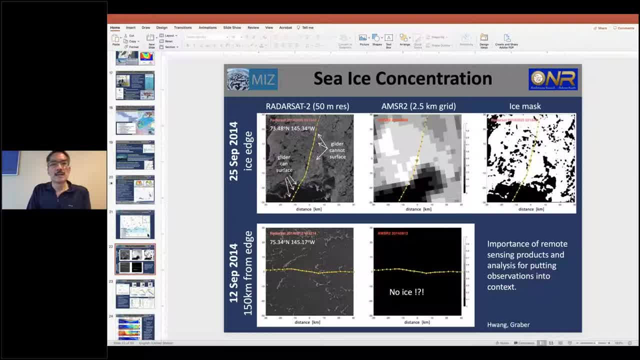 and it also gives you an idea of how how deceptive the remote sensor can actually be, where, if you looked at the radar side images, say from from mid-september, you would think there wasn't really any open water, but in reality there was enough open water for the glider's surface. 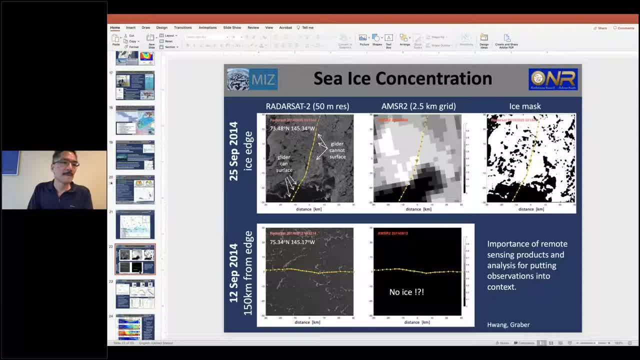 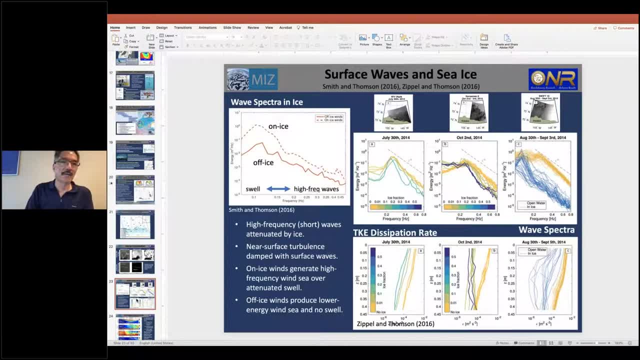 most of the time. so the sea ice perfection was was lower than you might have expected. so quick overview of some results. i'm a half hour in now. um, this is looking at surface. what one of that surface was one of the one of the things that we hypothesized. 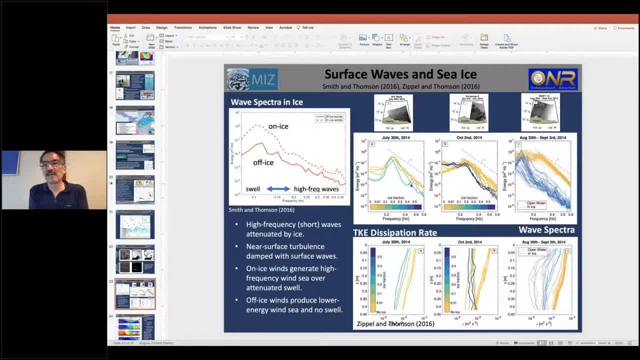 going into this was that we would see increasing surface wave activity and that would penetrate into the marginalized zone and really be affecting a mechanical breakup of the ice, so accelerating the breakup, but instead what you see if you look at um, if you look at surface wave activity in terms, as a function of frequency, so this is wave spectrum. 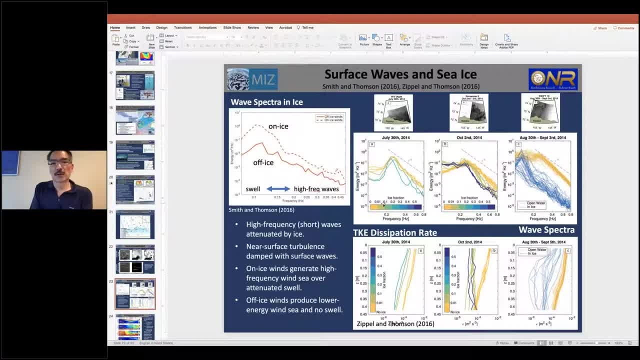 as a function of ice fraction, where the oranges are open water and as you go to increasing blue, those are increasing amounts of ice. what you see is that the um, the ice essentially dampens high frequency surface wave activity and there really wasn't that much low frequency. 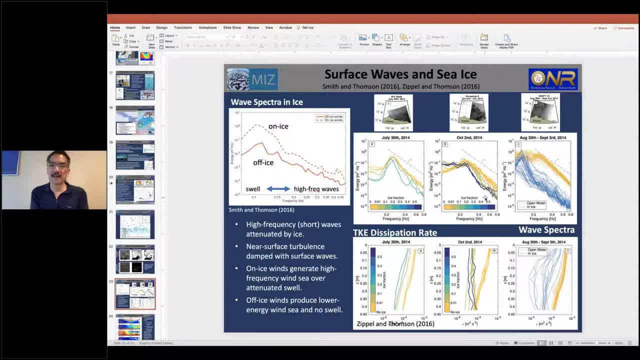 surface wave energy. so this is the ice was in a sense protecting itself. the marginal, marginalized zone, the lower ice fractions were absorbing the surface high frequency surface wave activity and preventing it from propagating deep into the ice. you see that in turbulent dissipation rate in the upper meter cell of the 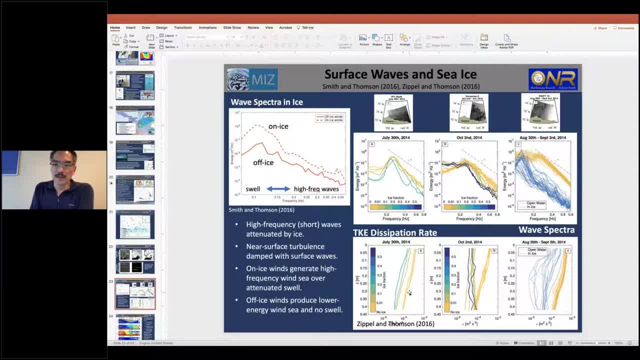 of the water column, where you see in open water a fair amount of turbulence and and you don't really see that in even small fractions of of ice cover. so the message here was that no, the ice is damping the high frequency surface waves. it's not propagating into defect breakup of. 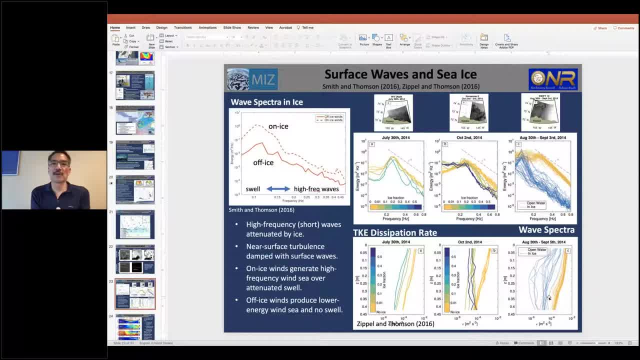 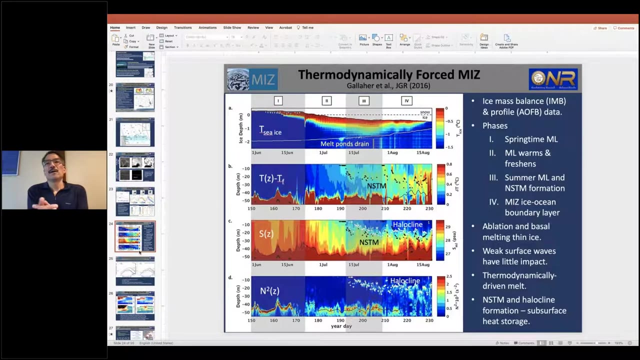 ice inside the marginalized zone. we don't yet see a long period. um low, low frequency swallow would propagate deep into the back, sort of like what you see in the antarctic right, where the long periods welcome, propagate deep into the back ice and effect breakup. so at least at this time we don't see surface waves having a large impact. what we do 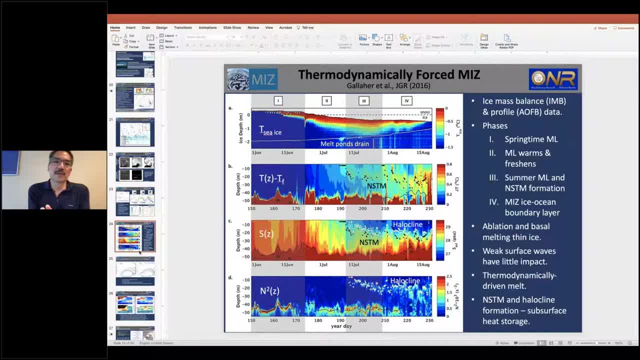 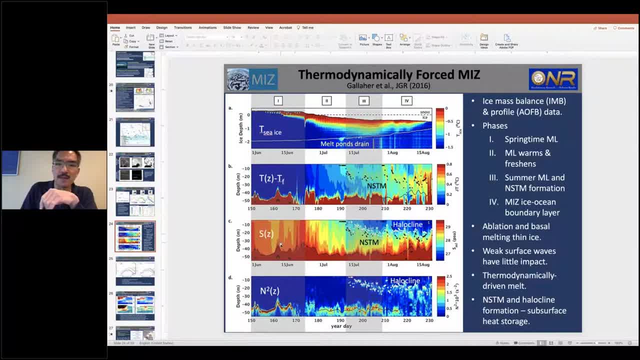 freezing point of the upper ocean and the salinity of the upper ocean and buoyancy frequency. so you see, uh, three phrases, three phases. one here, which is the springtime mix layer, we don't really see very much happening. you see the start, the ablation at the top right, just surface melting. the period 2: 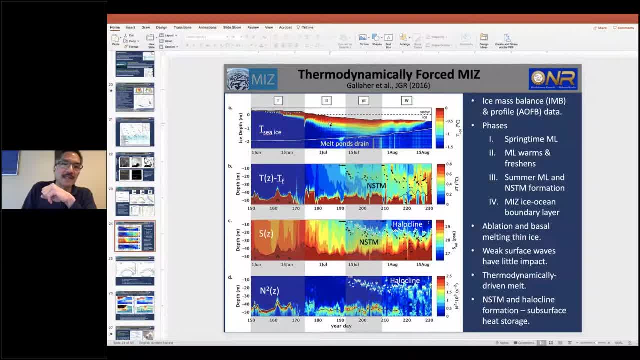 when you see the mixed layer warming and freshening. so ice is melting both from the top and basal melting is starting from the bottom and you see this freshening of the surface layer during period three. you've got enough open water that you have solar radiation penetrating. so you 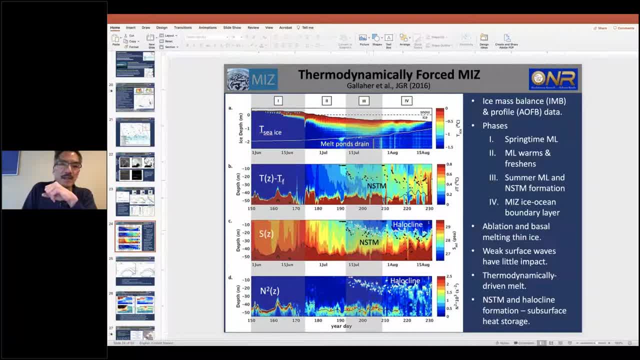 see the formation of this near surface temperature maximum and the development of a halocline which is isolating that from the surface. again more surface melting and then period four when you have a true marginalized zone, and then period four when you have a true marginalized zone. 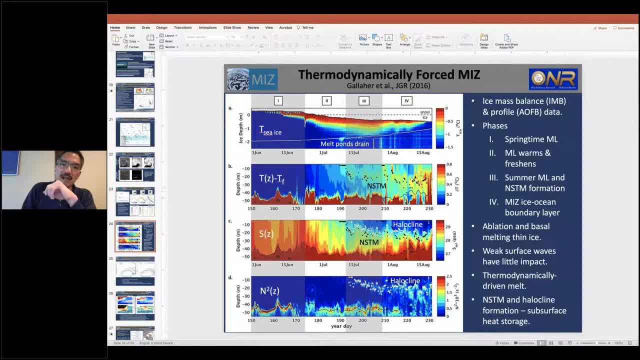 and an isocean boundary layer. you've got a very nice halocline developed and you've got this this trapped summertime heat in the surface layer. but again, the message here is that, no, we're not seeing the, the waves propagating and forming it, a mist like you would see. 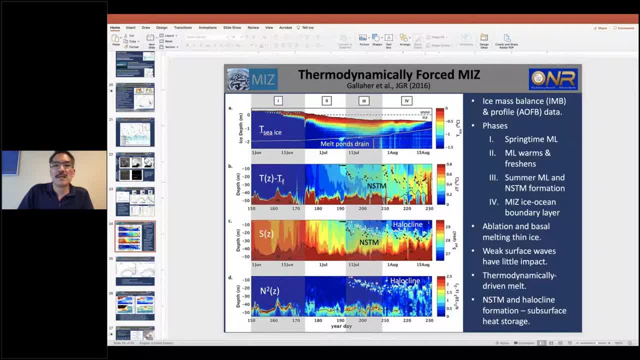 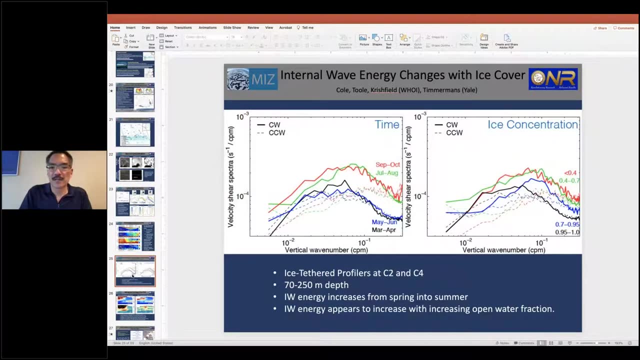 in the greenland sea or in the antarctic, but instead you really see this thermodynamic marginalized zone. so surface melting primarily, and some basal melting, and then period four. a few weeks later you have flat ГдеpMI states, Tokyo and blacks, versus periods when there's not much ice. you see increasing clockwise internal wave. 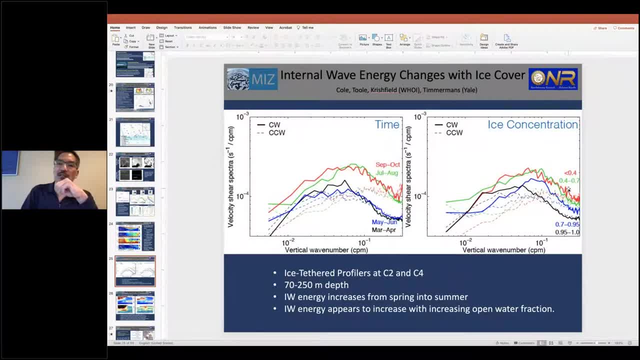 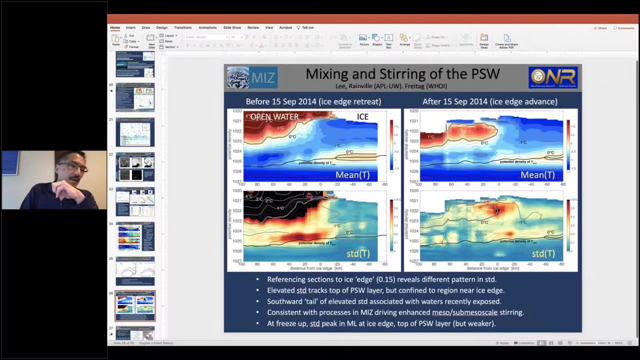 activity. so you see increasing downward energy propagation in the internal wave bands. so we're seeing what you would expect, which is more surface generated internal wave activity property getting in the interior and presumably generating more mixing. and the last bit of result from the uh, the marginal isome program, is signs of stirring mixing at the pacific summer water. here you see. 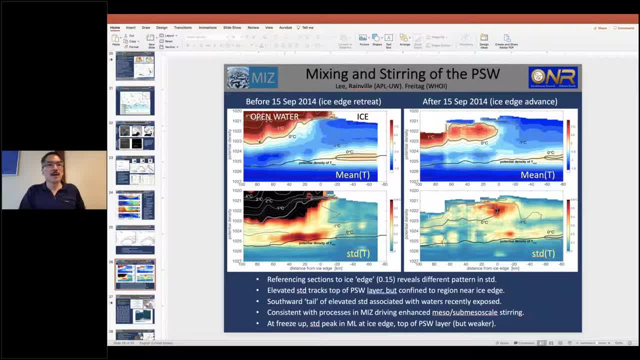 mean and standard deviation of temperature on isopicknels, um before the, the eyesight retreat and during the eyesight advance. and the thing i'd like to point out here is these are from gladiator sections and moving back and forth um into the back, from water into the pack and it's 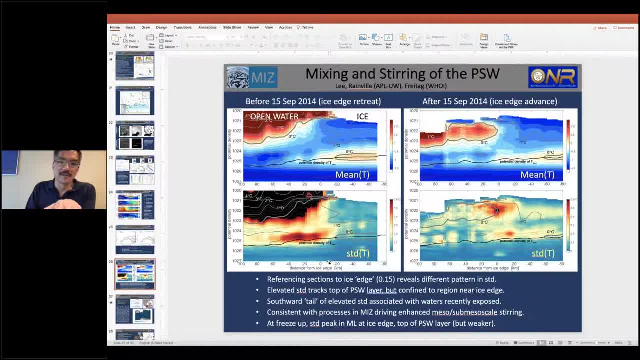 referenced relatively ice edge, where the ice is defined as a 0.15 ice concentration. so not much ice at all, really for the ice edge, but but you see an increase in the standard deviation of of temperature at this area that it's associated with the uh, essentially at the top of the pacific summer water. 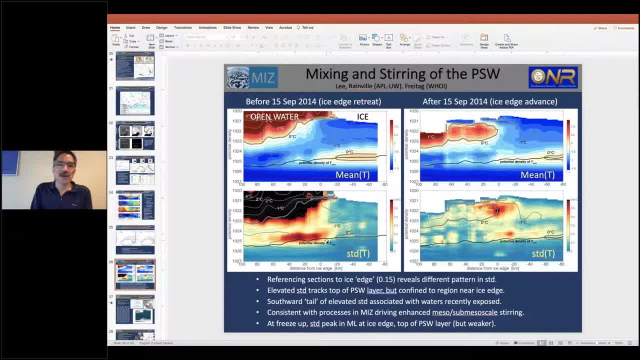 and you see that um very strongly during the ice edge retreat, less strongly during the advance. so here you're. you're essentially moving nice backwards um, the ice is retreating. you're seeing an area that hasn't really been written on by the atmosphere, whereas here, as it advances, this 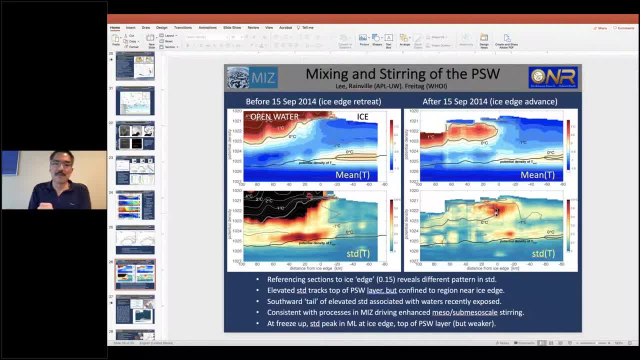 has all been- uh, been- impacted by atmospheric forcing- some mixing if you will, but but that southward tailed ass is is a clue that we're starting to see um signatures that we would usually associate with with stirring along an isopickle right that enhanced variability along 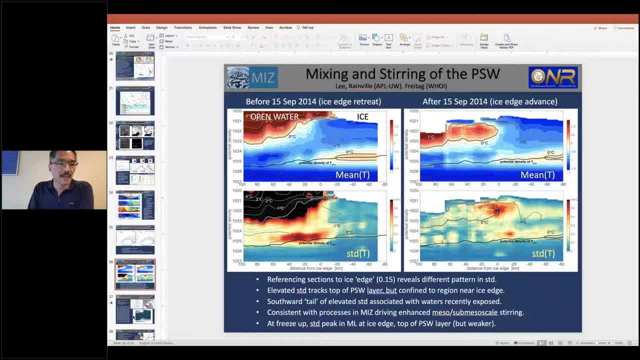 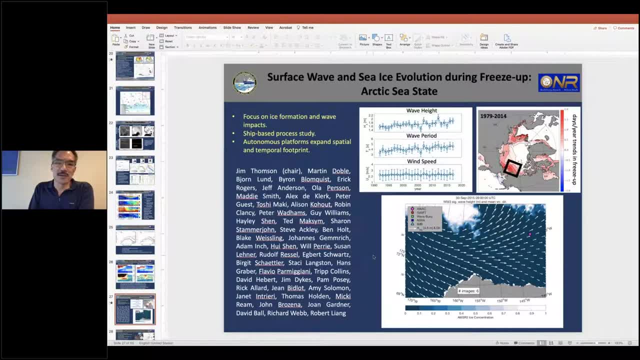 that is a victim. so i'm not really going to talk about the the sea state program. they've generated a beautiful volume in jgr- never encourage you to go look at that- but fundamentally that they were driven by this idea that if you look at the, the trend and freeze up, we're seeing a lengthening 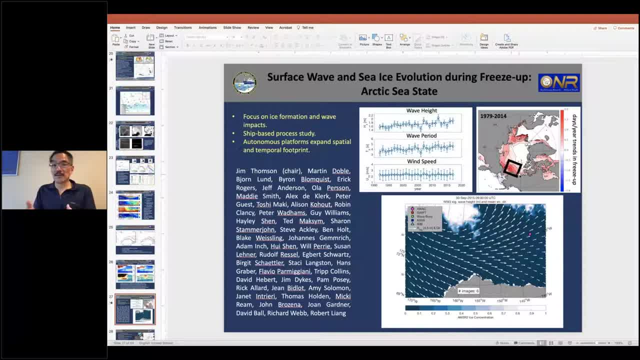 of the ice free period and that's been driven at both ends, but in particular it's been driven by an increasingly late freeze up in the beaufort sea at the same time that you see increasing segment wave height, increasing weight period in the beaufort at that time of year. so the the thought 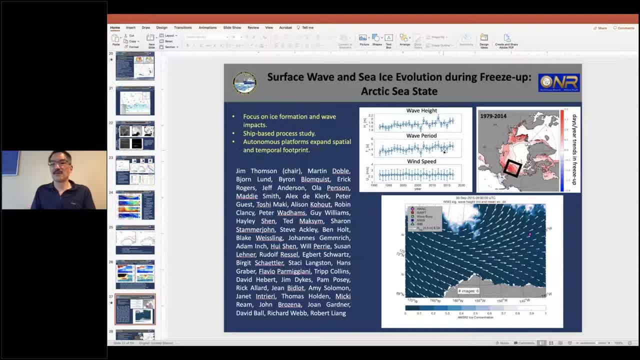 is that you see an increasing impact of the surface where generation in? in driving, uh, in driving the freeze, the freeze up into a later period of the fall, and that's uh. that's by extracting heat from the near surface temperature maximum, perhaps on the pacific water layer. 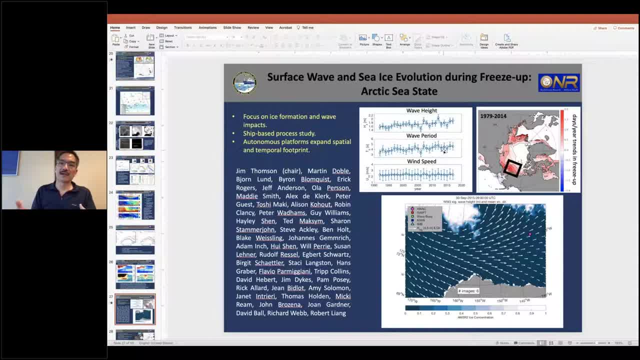 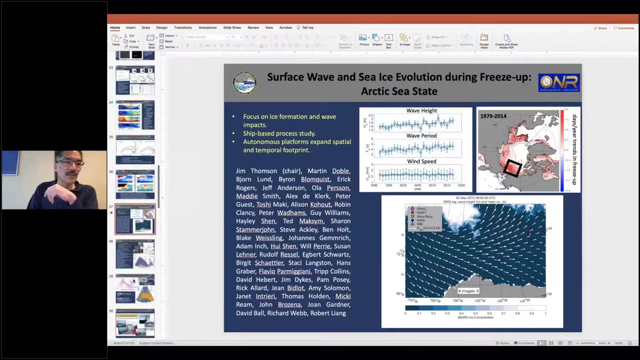 and also by by this mechanical activity that changes the nature of the ice that's forming. you're seeing an increasing amount of pancake ice versus other ice types, say frazzled formation and formation to uh feather ice types through the through the winter. so just in the interest of 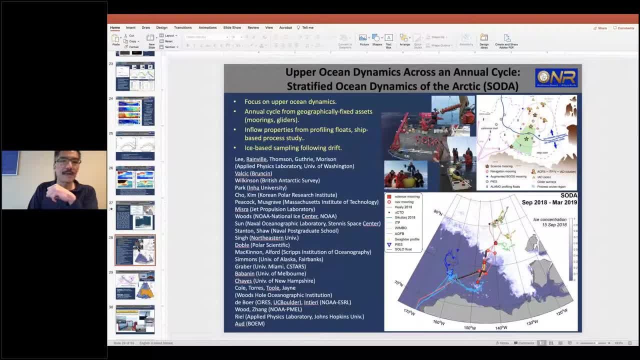 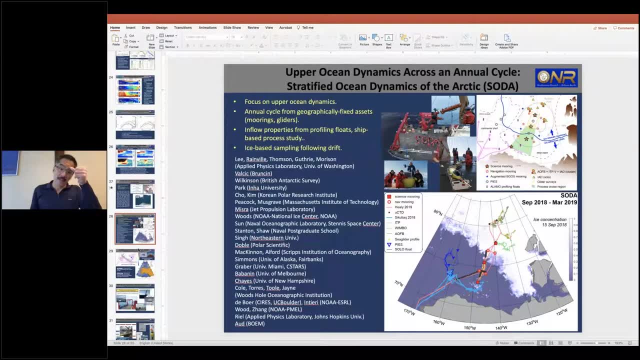 time i'm not going to focus on that, but it really is worth looking at. the sea state program has really, really been produced, producing effective results. ultimately, we have done a great job also of producing a lot of fantastic results. so, lastly, i'd like to move on to the stratified ocean dynamics program. 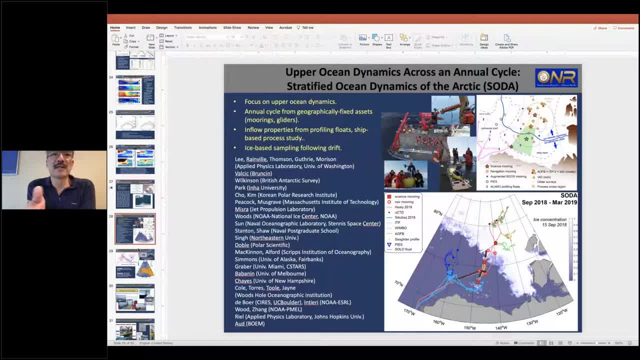 and this is the analysis- that this data is still in progress, but here the goal was to focus on annual cycle right to look at the entire year. so we look at season, look, try to look at seasonality over the course of the year framework so that we could see contrast as we look towards areas. 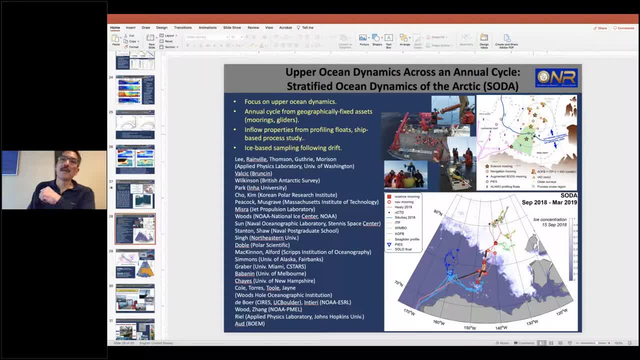 If you look here, the stars are mooring, so the southernmost mooring is an area that sees dramatic changes, nice cover, over the course of the year. The northernmost star is an area that is really under the pack, either the entire year or 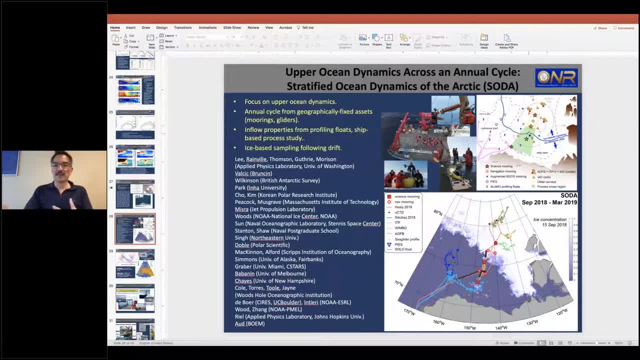 at least most of the year, And that middle one is in the area that sees a lot of marginalized zones, so quite a lot of contrast through the year. There was also acknowledgment that the incoming Pacific water was a huge player here in setting what you see, and so a focus on looking at the Pacific water inflow. 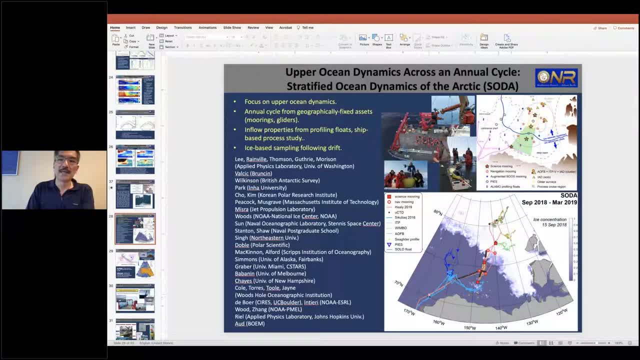 A split between a process cruise on the Skoliak during the summertime looking at Pacific water inflow and a variety of assets on the ice and moored to look at the annual cycle, And again an enormous team of very talented people looking at a broad range of assets. 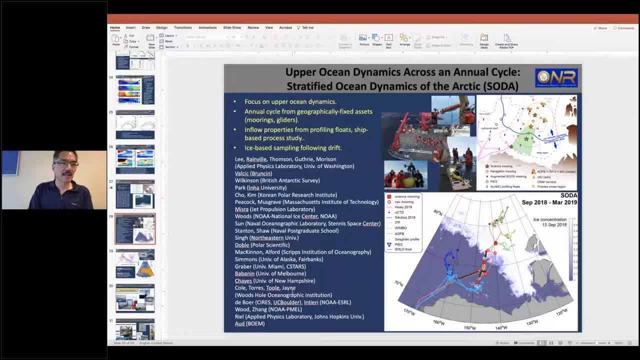 A broad range of activity there, a broad range of the science, And one of the hallmarks I'll talk about was there was an attempt driven by the Office of Science and Technology Policy at the present to make this a broad interagency program and to see how far we could get by expanding the activity out. 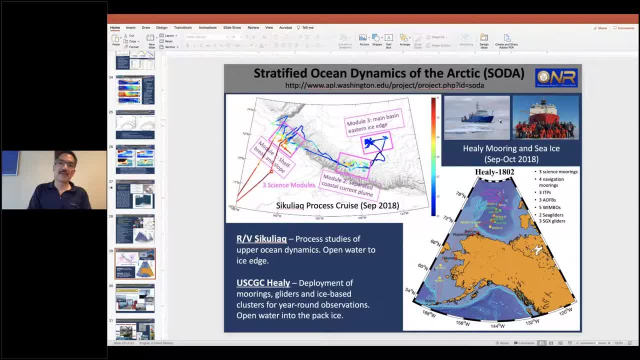 So cruises a lot of ship-based works. The Skoliak went out for process studies and Healy went out twice To deploy more in ice-based assets than to recover them, As Skoliak divided the work up into modules. looking at the shelf break and slope, looking 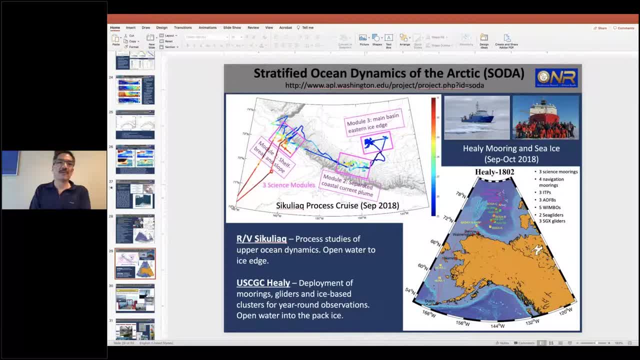 at an area where you see these plumes of Pacific water separating off and moving offshore. then looking at the mid-basin, at the ice edge, where Healy really focused on the deep basin, Looking primarily deploying assets but doing some process work with an underway system. 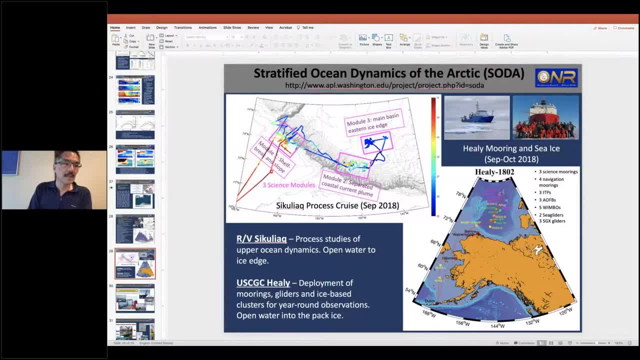 So that's what we're going to talk about in a little bit more detail in just a few minutes, And then we're going to talk a little bit more about what we're going to do in the next few minutes, And then we're going to talk a little bit more about what we're going to do in the next. 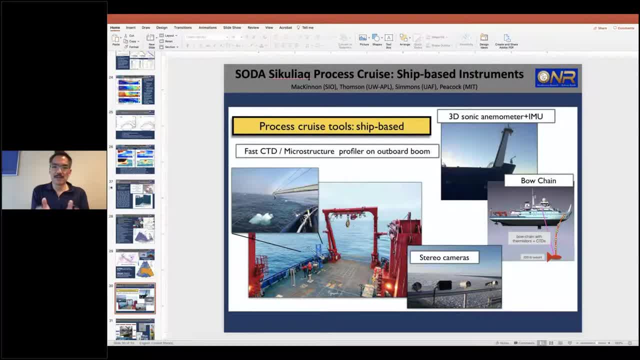 few minutes. So Skoliak is particularly interesting. It was led by Jen McKinnon And she really put together this cruise that did process studies the modern way, right Where you have a variety of intensive process-based measurements from the ship, a very fast CTD. 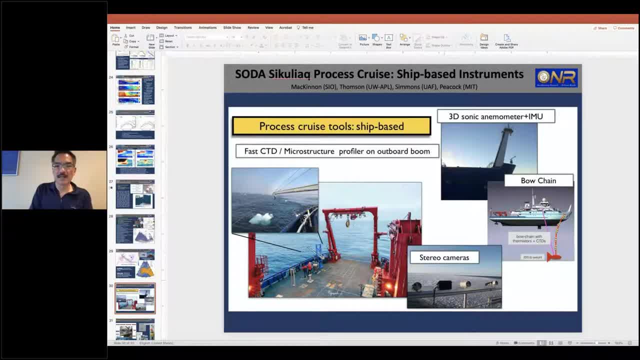 intensive meteorological measurements: boundary layer met stereo cameras looking at the ice and a bow chain looking at undisturbed upper ocean water column right from the bow of the ship but then expanding that footprint out right. So the way we do these measurements these days is you take the measurements from the 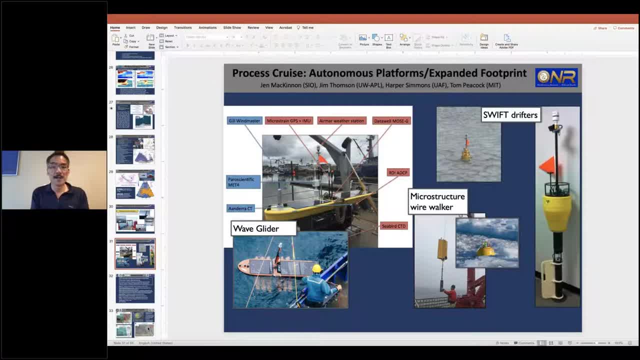 ship, but then you deploy an array of autonomous instrumentation around the ship to expand the footprint, to do things in places where the ship is not and just in general, to take measurements that are very difficult to collect from the ship. So they had wave gliders. 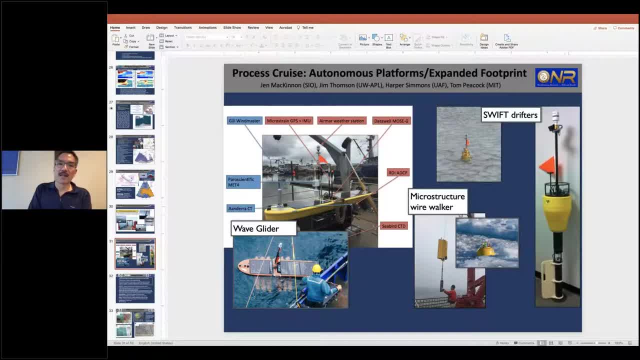 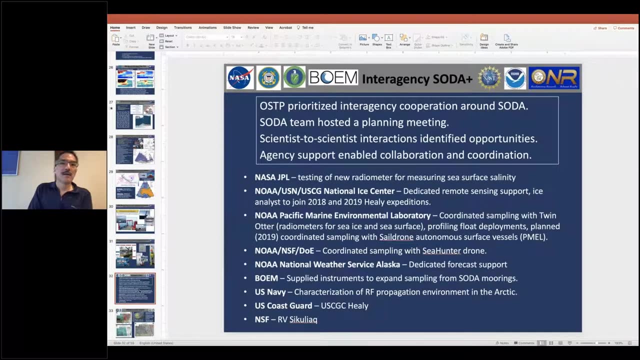 Making measurements around the ship. They had a variety of GEMS surface drifters making surface-of-wave measurements around the ship and then a wire walker drifting around profiling the upper part of the water column and making microstructure measurements. So beyond that, there was this push to make an interagency SOTA, and that was NASA Coast. 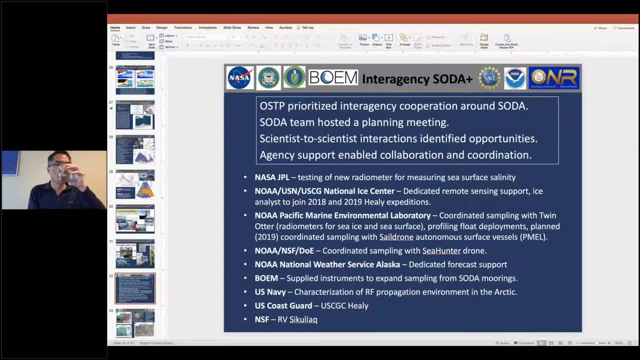 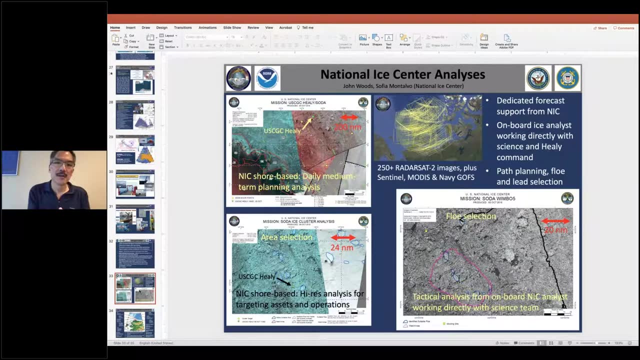 Guard, BOEM and NOAA NSF National Ice Center, So a large number of collaborators, and I'll focus on just a few of those at this point. As I said before, remote sensing is key to a lot of what we do up on the ice. 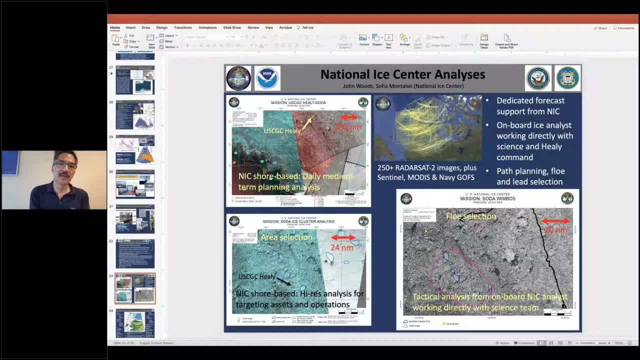 In this case, we had dedicated analysts from the National Ice Center sailing with us. Sophia Montalvo sailed with us. John Woods coordinated a lot of this. What I meant was that we got a continuous feed of very high-quality imagery from the NIC. 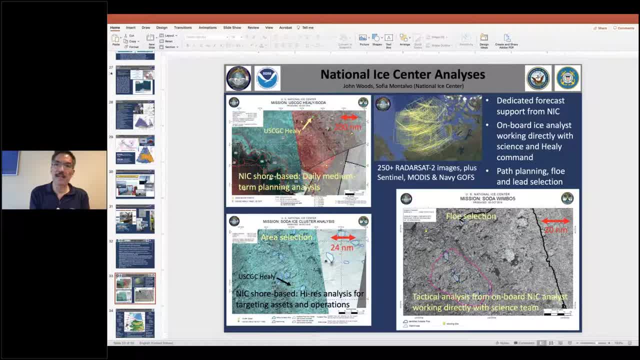 Shipped ashore, Got it. We got in both Sikuliak and Healy And that imagery was archived for use in the science analysis afterwards. But that tactical analysis allowed us to target what we did at sea. We could find these large multi-year flows which you see circled here and drive to them. 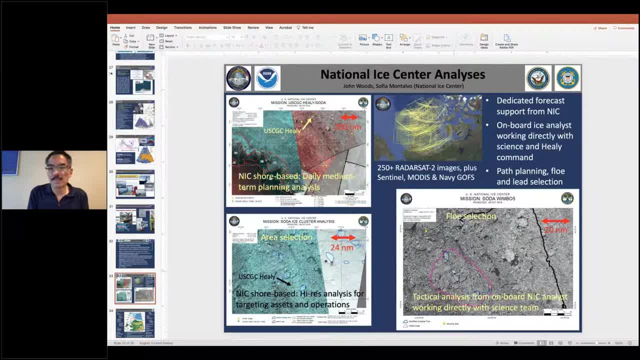 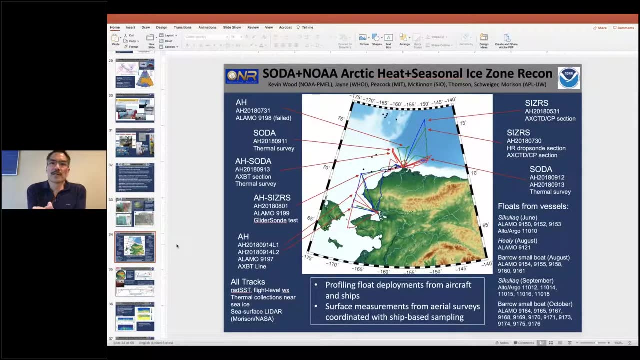 to put instruments out on the ice. We can navigate efficiently through the pack, So very, very critical, both for science analysis, Yeah- And for operations. In addition to that, we had a collaboration with NOAA, Taquit and CISRS, the Seasonal 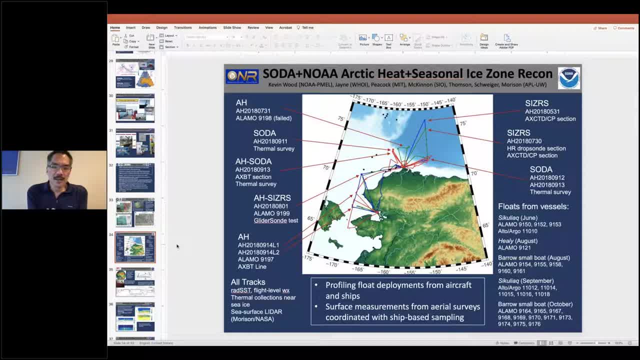 Livestorm Reconnaissance Program to make a variety of flights. You can see lots and lots of aircraft activity dropping both expendables and Alamo profiling floats into the Pacific inflow and into leads around the ice. So these are all great because they allow us to track Pacific inflows. 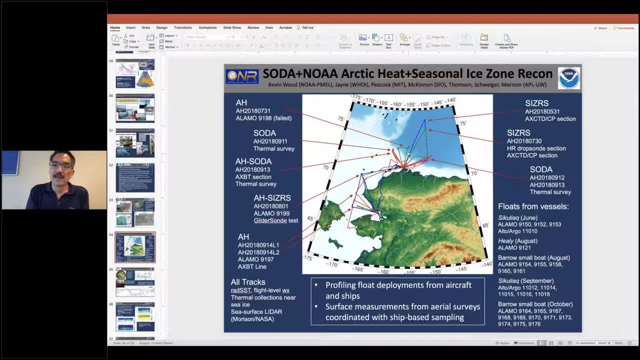 So these are all great because they allow us to track Pacific inflows. So these are all great because they allow us to track Pacific inflow properties as the floats get carried along the inflow. They also allow this broad look at what the scope of the Pacific water was during the 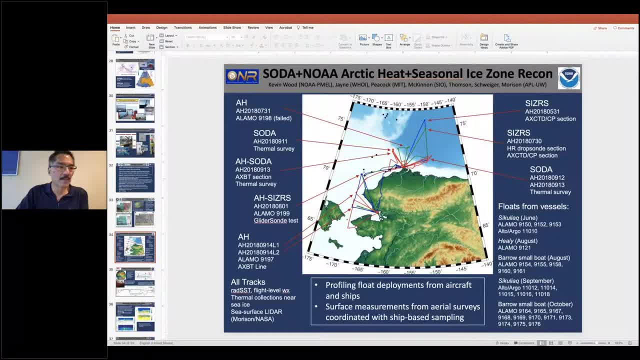 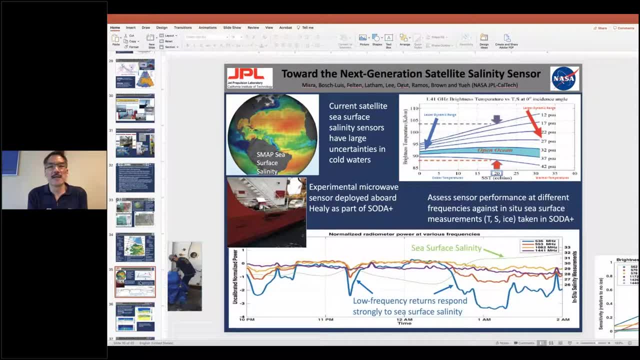 course of the major fuel program during the SOTA campaign. I threw this in here because it was interesting. We had a group from JPL, the NASA board, who were testing a new salinity sensor Right. So the driver here was: 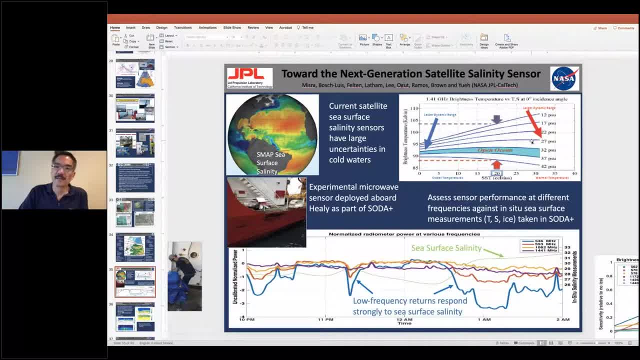 They're learning how to do salinity from space, and we're getting very nice results from that in the global ocean. But as you go into colder waters, the dynamic range of that sensor gets very narrow, And so they need to learn how to use that sensor in Arctic environments. 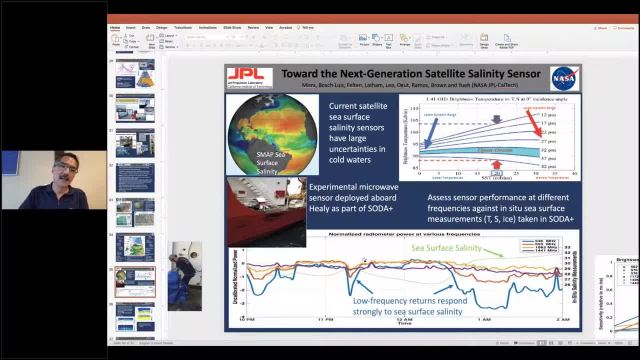 In order to do that, they mounted a radiometer from Healy as we drove around, collected measurements at a variety of different frequencies and looked for different frequency bands where they saw a particular response, Right Where they could see signatures that they could relate to changes that we saw in the 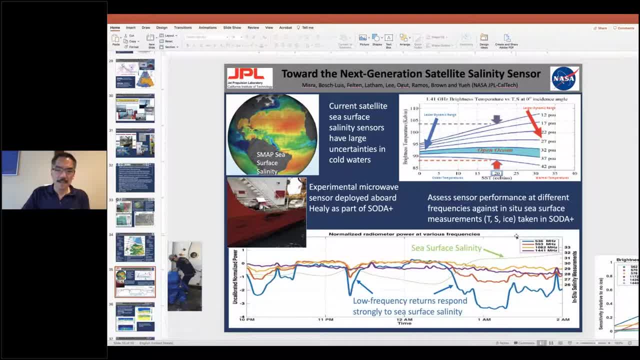 intake temperatures. That was successful in the first iteration In 19,. they weren't able to get things together well enough to come out again and the subsequent crews were hoping they'll come out again in this coming year, in 21,, when we go out to. 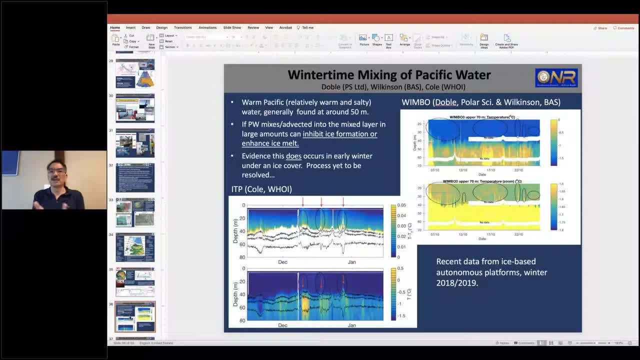 continue testing that sensor. That would be a huge advance if we do. salinity from space in the Arctic, in the open waters. So, to wrap up, I just wanted to show you some early results, some things that we're seeing from the SOTA data that people are pursuing in analysis. 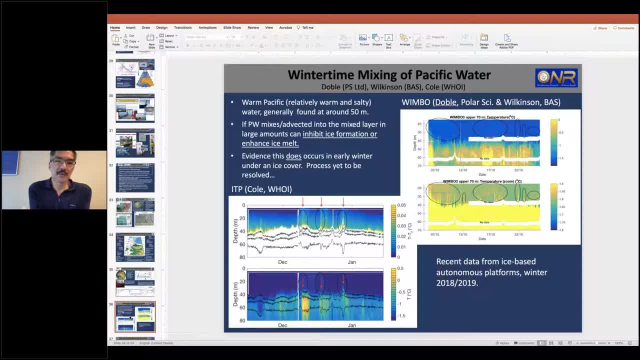 These are results from a couple of the ice-based instruments that were drifting around in the central part of the Arctic. So these were deployed pretty far north as part of SOTA and drifted south. But interesting, what they see over the course of the winter time are these injections of. 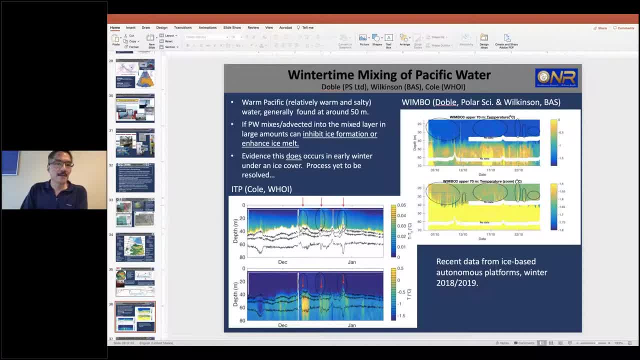 Pacific water Right. So they're seeing these what look to be mixing or upwelling events, where they see warm water being brought to the surface during times when we think that there's pretty extensive ice cover Right There might be. we're trying to figure out if there were leads, if the ice was more mobile. 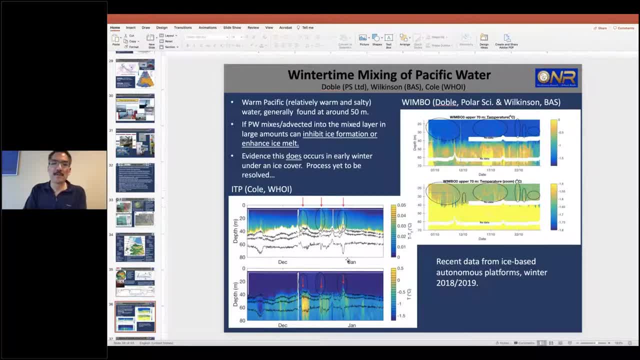 during these times in winter periods. But we see these events in data from multiple instruments, So it's not just a single instrument, they're fairly commonplace. So trying to understand that wintertime injection of Pacific summer water into the water column. 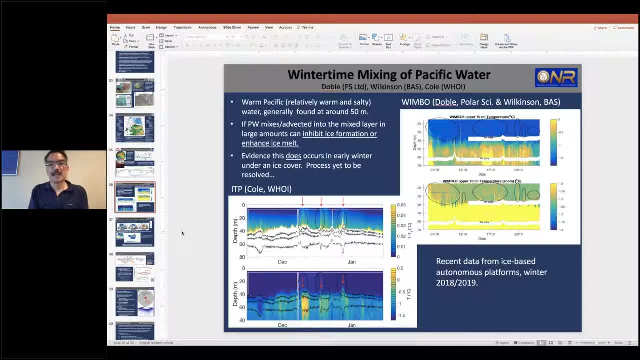 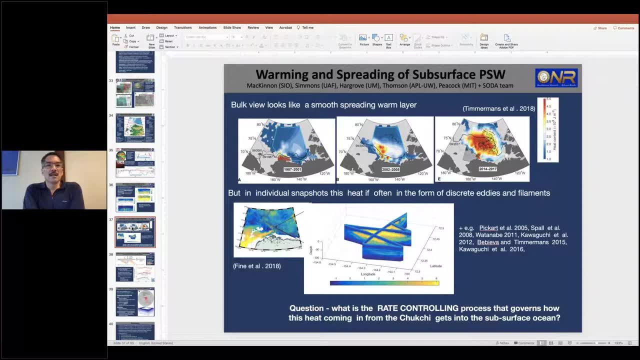 into what role they may play in weakening the ice cover, in maintaining or forming leads or enhancing early ice melt. These are results from Jim McKinnon and Company, from Sikuliak and the thing that they're seeing if you look at that top of the plot. 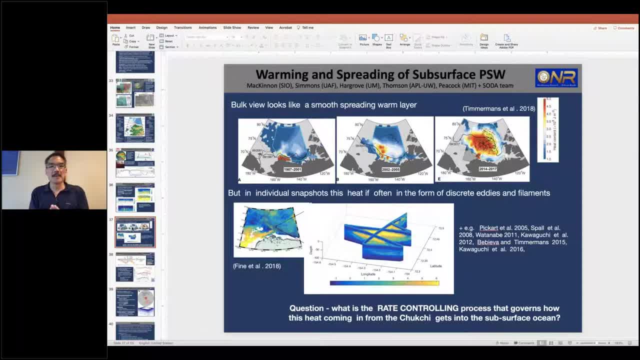 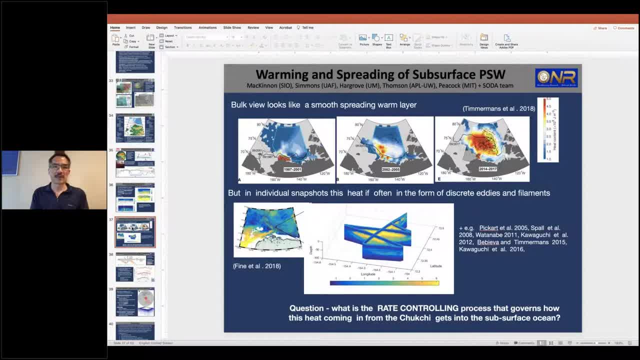 And that work is generally done from a variety of platforms. right, The available data is heterogeneous. It's from ITPs and from scissors measurements on pretty much anything you can get, And when you look at the spread of Pacific water from that lens, 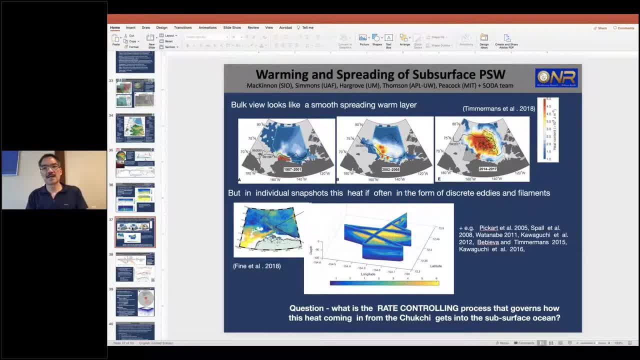 it looks like this widespread right, the generalized spread of warm water over the central Beaufort. But if you look at an individual snapshot, you look at something like what Jen and her crew did using Sikuliak. you see instead these filaments of Pacific water that come out. you know Pacific water comes. 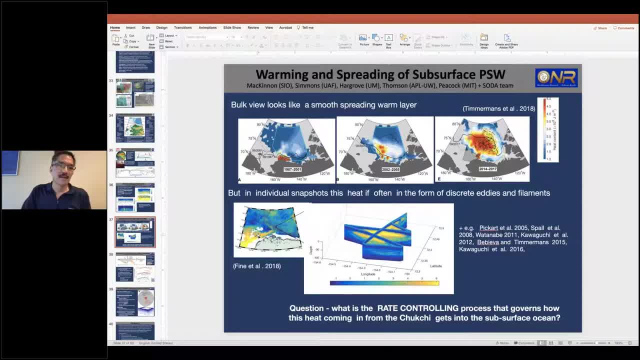 flows in the Bering at the surface, flows along the coast and then turns out, in this case, kind of around Bear Canyon right, which is one of the areas that Harper Simmons and others have been modeling and looking at as a major inflow site and subducts right. 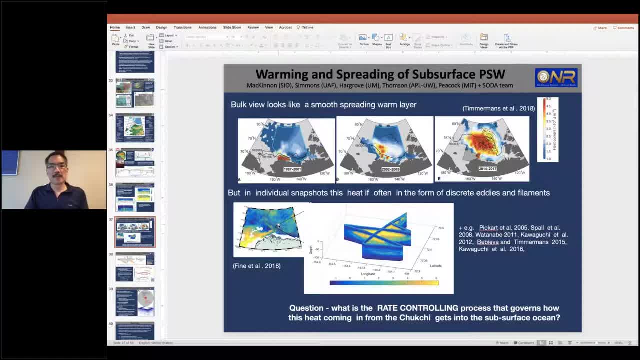 At this point it slides under the colder but much, much fresher Arctic water that's out in the central basin and to some extent disappears from view. So Jen sees a large event, right, a large filament coming out and subducting and is starting to ask questions about you know. 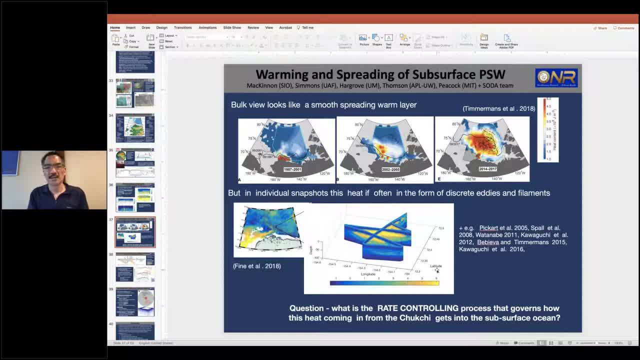 what controls the rate of these kinds of processes? right? Where do these filaments peel off the coast and enter the open basin? How often do they do that? right? How efficient are they at moving heat into the open basin, With an understanding that the actual mechanism that gets you to this upper row of plots is really 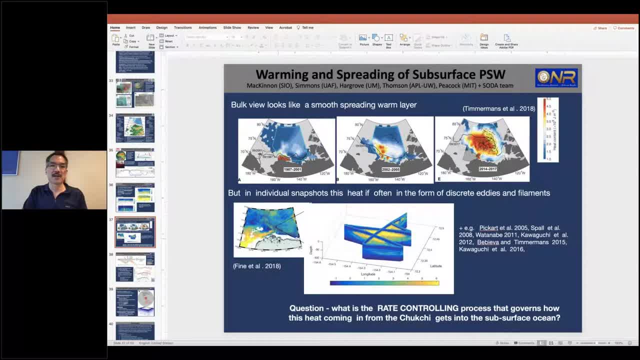 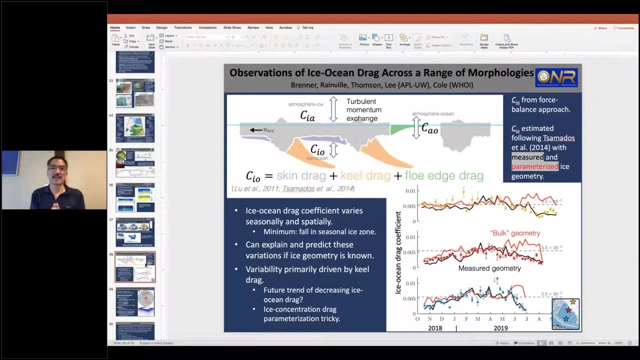 probably an amalgamation of lots of small-scale processes that look like this right Filament already formation and ejection from the coast, So trying to understand those dynamics. And then the last piece from SOTA that I'd like to leave you with is work of Sam Brenner. 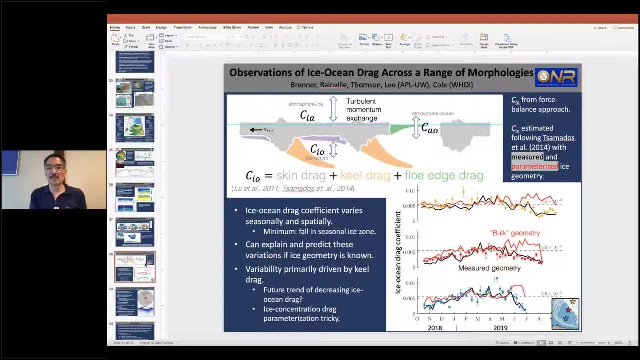 who is a graduate student here at UW. This has been recently published And Sam was looking at, as a first cut, at the mooring data: data from the moored instruments looking at observations of ice, ocean drag and the flow of the ocean and what, frankly, the feet are doing. 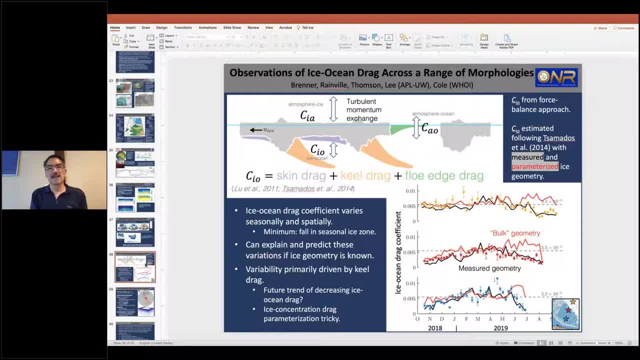 association drag and trying to understand the division of labor between skin drag, so the drag just on the surface of the ice keel. drag, so the drag associated with major keels and nice formation of roughness on the bottom, and flow edge drag right on the edge and 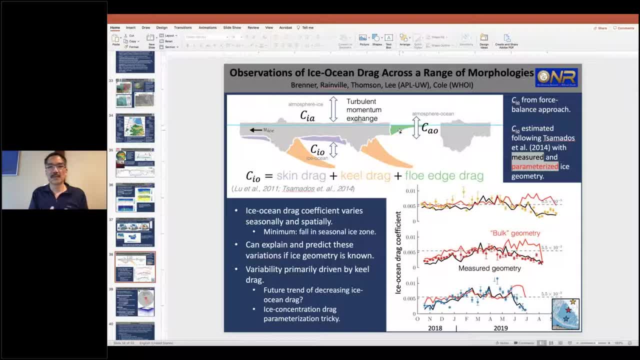 to understand how well the current models do in predicting that, And so he looked at three different areas, right the three different moorings, lots of open water, lots of marginalized zone, lots of pack, and tried to understand the difference in his ability to predict if he took the geometry that was measured from the insurance we have. 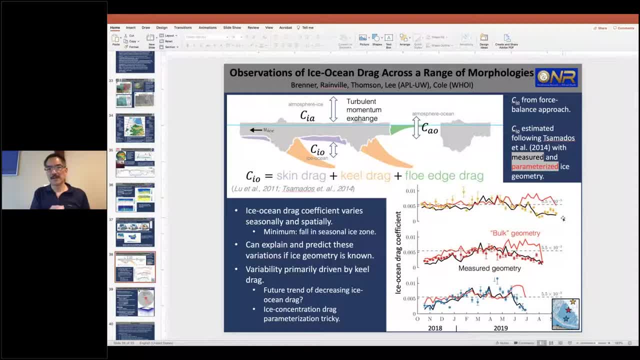 in the moorings. So we have measurements that can estimate the ice geometry, and so now you're not trying to parameterize the geometry, You're just parameterizing the drag, versus what happens when you don't really know the geometry, and you're trying to parameterize the whole thing. right, so you're say parameterizing. 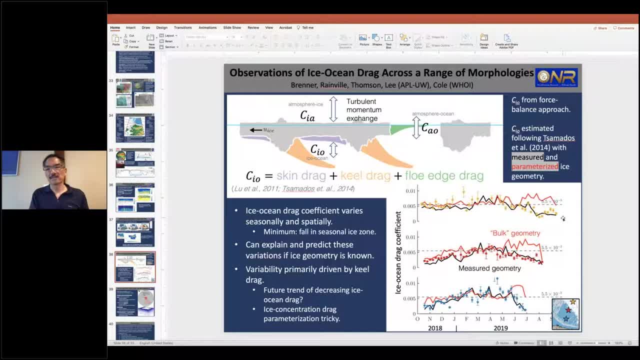 the geometry based on open water fraction and then parameterizing the drag from there, And the answer that he gets is that if we know the geometry, the parameterizations for drag work really well and most of the drag is in the keel drag. 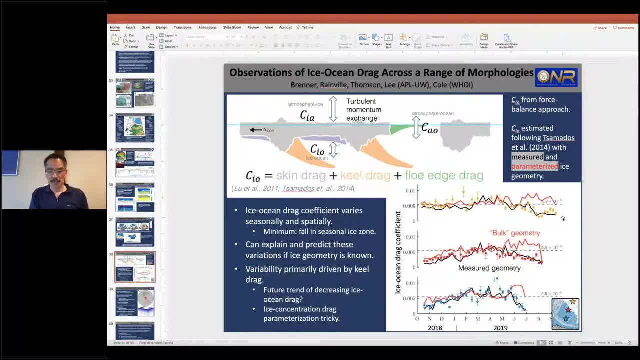 But if you don't know the geometry, the parameterizations for geometry that are based on, say, flow size, distribution or open water fraction don't do particularly well and therefore the parameterization from drag doesn't do particularly well. So that's where we stand in terms of being able to do these things for the models at. 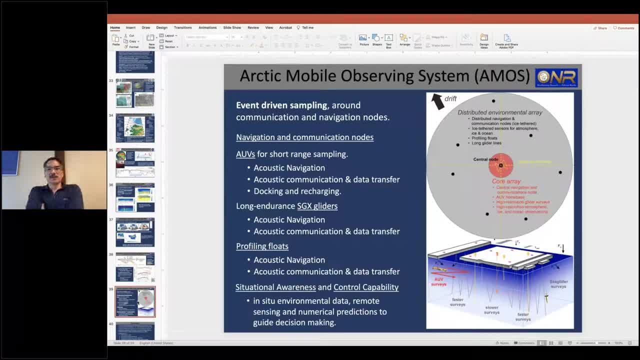 the current time. So I'll conclude with the next step, which is the Arctic Mobile Observing System program, Which is where we're at right now. We're currently in the second year of that program and really this is primarily a technology focused program, trying to develop the technologies that will allow you to do event-driven sampling. 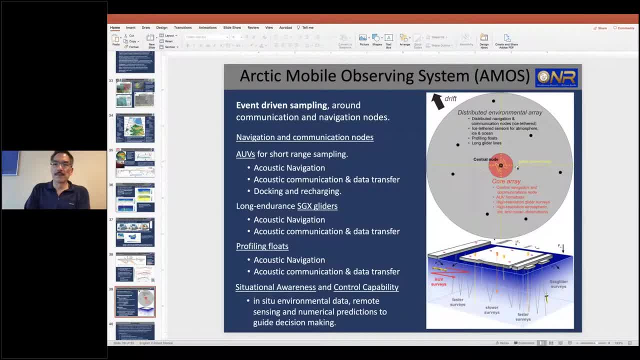 around the central node. So the idea that you'd have a large central node that was well-provisioned might support a fast, propeller-driven AUV that could dock at the node and be sent out occasionally for very short-range missions. You might have other platforms- ice-based platforms- distributed around the node. 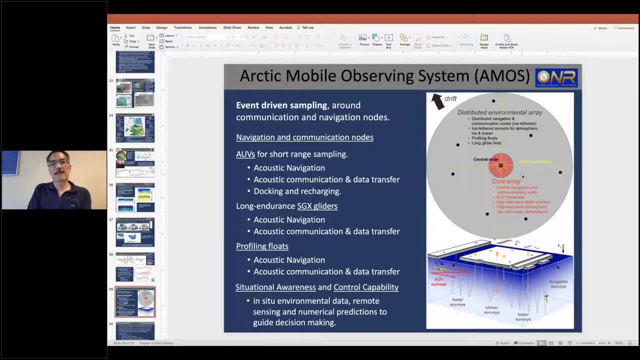 The combination of these platforms will provide acoustic navigation for long-range gliders. that will give you the ability to sample both closely around the node and range tens or hundreds of kilometers away from the node to sample the area around it, perhaps storing profiling floats. All of these things can be used for time distribution or time release into the area, so you could 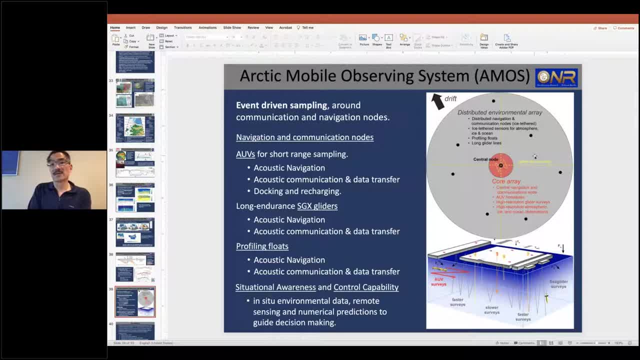 drop them, either driven by events or times, into this area and then they would profile as other profiling floats to at intervals, so they would eventually drift away from the node but would give you an intensive profiling capability for a while. And then you wrap all this up into a system where you've got 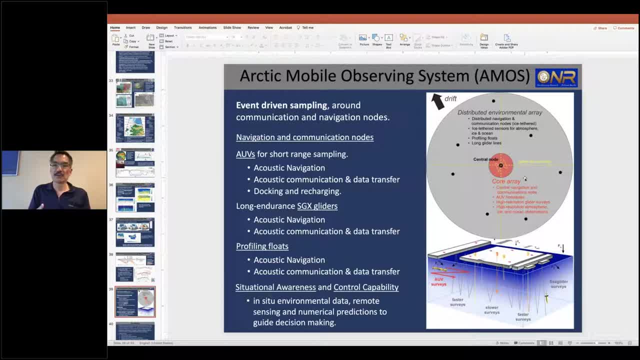 End some ability to bring the data back in real time, understand what's happening and respond. I control the system And you can see the little cartoon here of what we're trying to do, where the central node is actually a substantial spar. 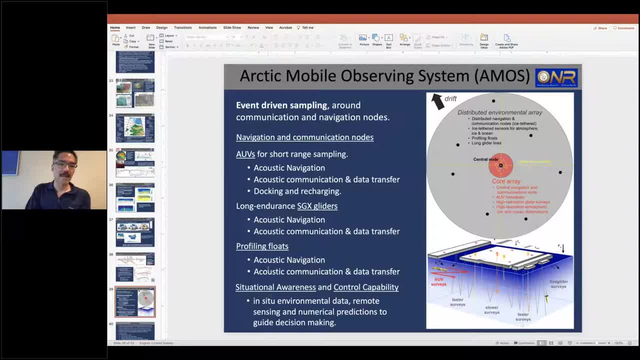 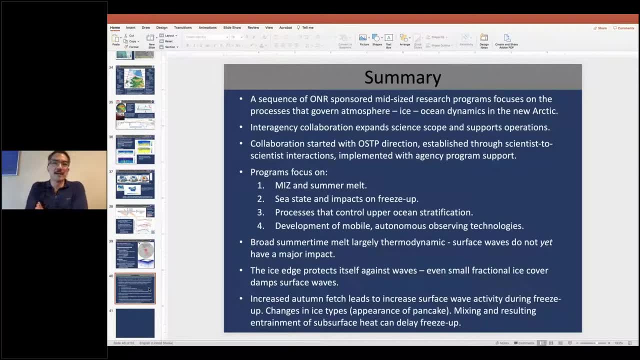 that's been more than the ice. So that is the current effort And I'll leave you with the summary slide there of where we're going. But again, this is a sequence of stage ONR research programs focused on the basic research, mainly on the physical part of the science. 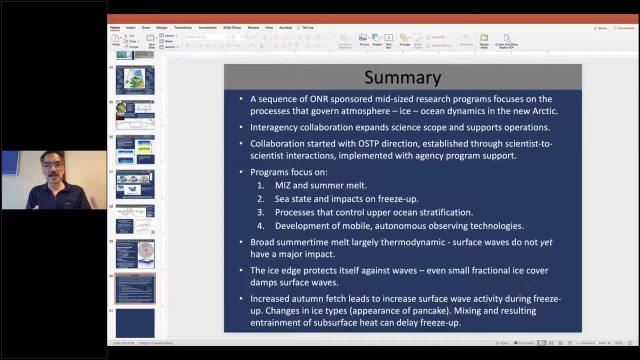 but you can see where the impacts might be for the biology and the biogeochemistry And a mix of understanding process level dynamics and developing the technologies that we need to maintain that persistent presence and access the space and time scales that are really of central. 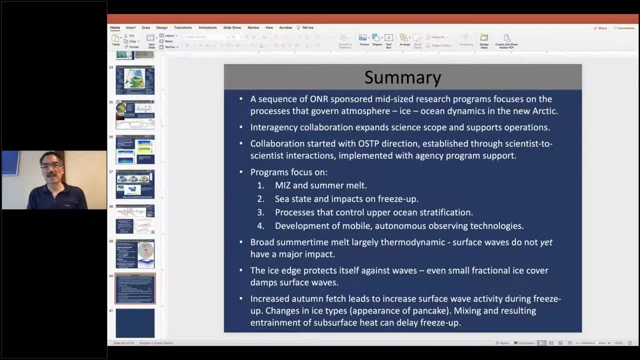 interest in our ability to to advance our understanding of both the physics and the tomorrow of the Arctic over a much longer period of time, in a much more distributed fashion. Thank you, That's all I have. Awesome. Thank you so much, Craig. 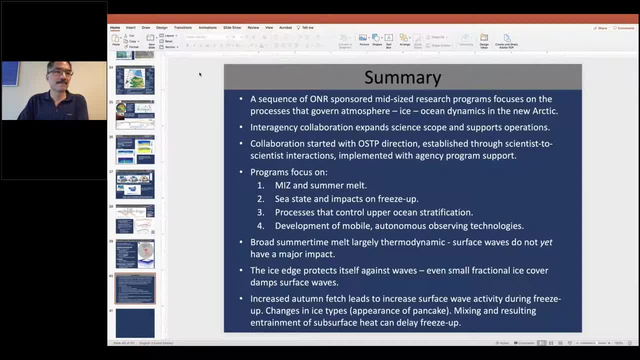 Just going to turn on video really quick. Thank you, That was. there is a lot to do in that program. It's been going on a lot longer than I than I realized, especially starting with MIS program, So I'm just going to go through a couple of the questions I know we only have. 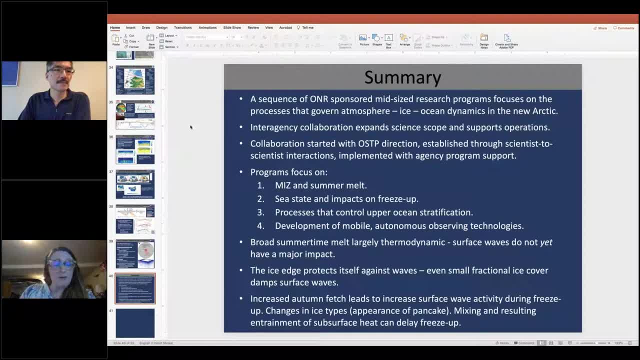 a couple minutes and you have to leave right at 11.. So I'll start with Libby's second question, actually, which was why was the Beaufort Sea the focal area for the studies? A couple reasons, You know. if you think, from an Arctic impact standpoint, the Beaufort has really 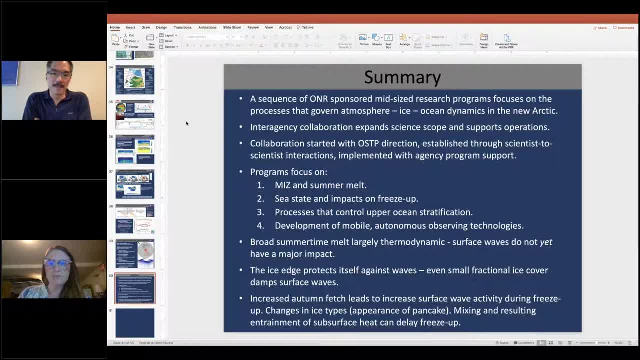 been the focus of a lot of our thinking. right, It's a freshwater reservoir that we think breathes in response to atmospheric forcing, So it's potentially the source of a major freshwater release, which may actually be underway right now. It's part of the work we're doing at 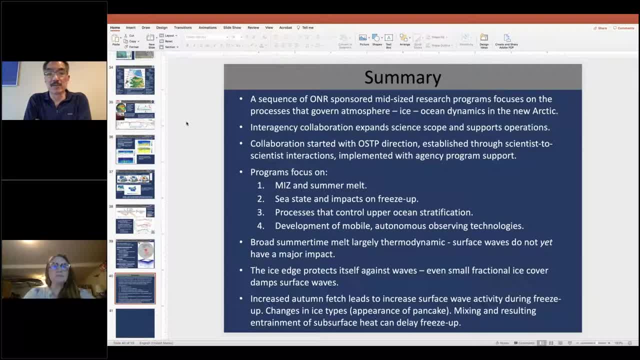 Davis Strait. It's an area of interest to the Navy and it's an area of interest to the US from both the national security and from a human activity standpoint right. It has an impact on our Alaskan communities And it's also a very convenient laboratory. It's a place 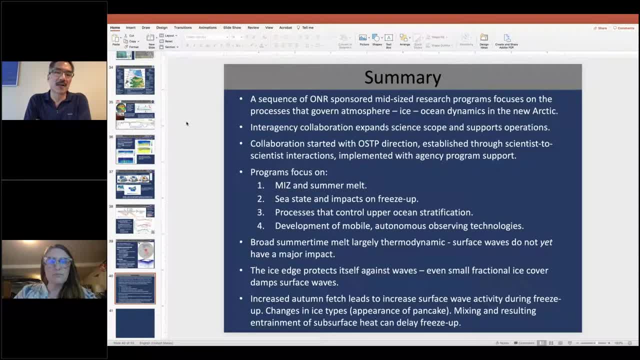 that we can get to fairly easily and has the right range of dynamics and ice types that we would like to focus on. Thanks for that. Craig Chidong also had a question. A major challenge of observing the MIS is to have co-located data of the upper ocean surface, with or without ice, and the atmospheric boundary. 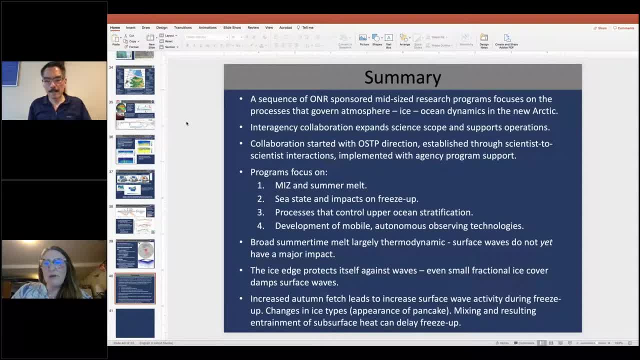 What technologies are out there that may make such co-located observations possible? So that is indeed the problem with the MIS. One of the elements of the AMIS program is a large- and I really do mean large- spar buoy. I didn't throw a picture of it in the diagram, but it's large enough that we can. 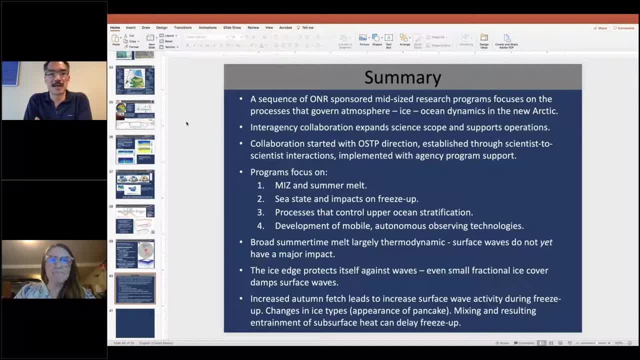 only carry a couple of them on the ship at a time for deployment And it's meant to survive, freeze up and melt out pretty routinely. One of the things we're using it for right now is a testbed for boundary layer measurements. My thinking about that is a testbed for developing the kinds. 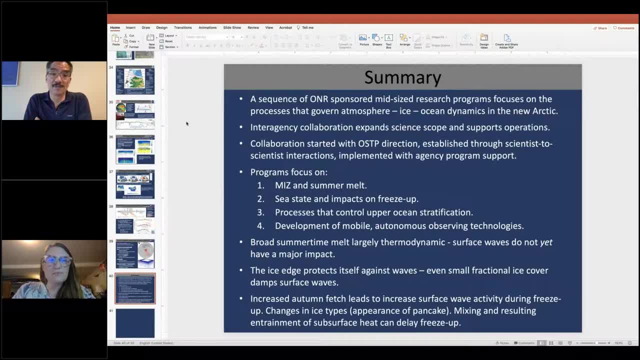 of technologies. we need to make these measurements untended from high-space platforms over long periods of time. But because the platform is a bit of a brute right, it gives you that ability to hang out in an area, almost no matter what's going on, and collect those meteorological measurements. 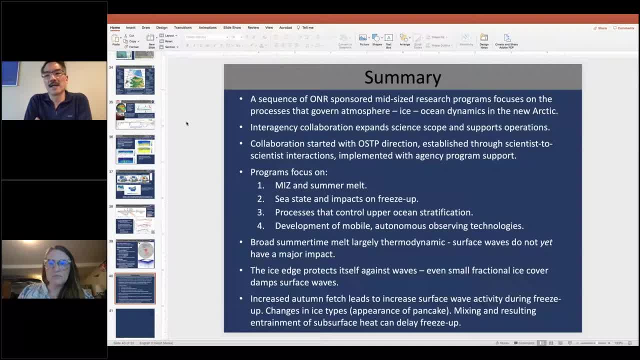 So the combination of that and the ability to have mobile platforms, gliders, AVs, floats in the water column gives you atmosphere and ocean, And for the ice it's harder right? Yep, you just have to rely on things that you're they're going to die over the course of making. 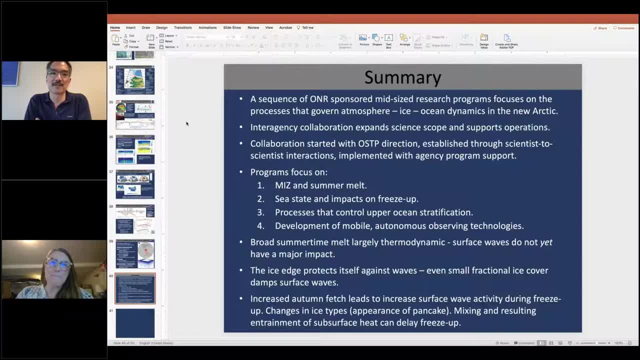 their measurements and make them cheap enough and that they can be put out in great quantity. that's a hard thing to come to grip with, of losing, losing something you've made. yeah, we're good at that, though, at losing things, trying to understand how to make them so that we can use them. 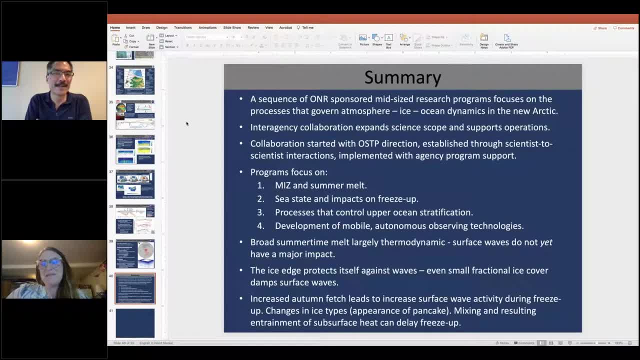 right, yeah, doesn't doesn't always make it any easier, but yeah, um livy had another question which i think we have time for. it seems um, and this goes back to your um early slide on, like the time scales and sort of the applications um, where that has um she says it seems the. 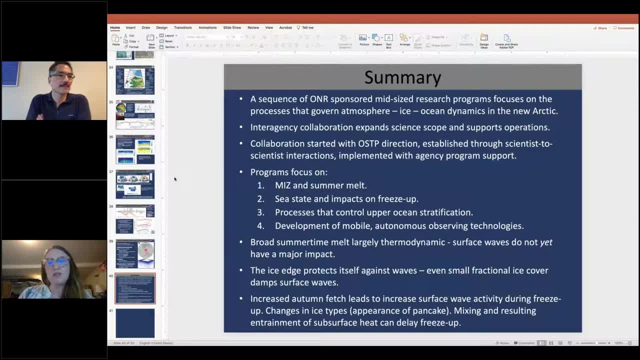 intermediate scale of strategy might be the most challenging to achieve. any thoughts on that. um, you know, the, the strategy and the climate scale are not terribly different from each other, i think, in that they, they nest pretty well. um, you could think of the, the strategy scale as. 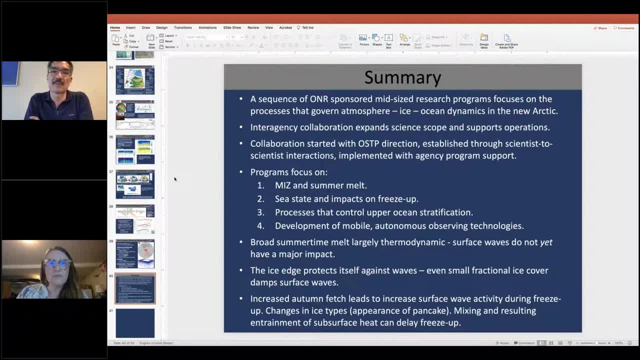 as doing more of what you're already doing at the climate scale in areas of focus, say, um, you know, if you- you knew you wanted to- to make predictions of of ice or out of ice cover on a annual, inter-annual time scale. you might concentrate measurements in the areas where you think shipping activity was going to.